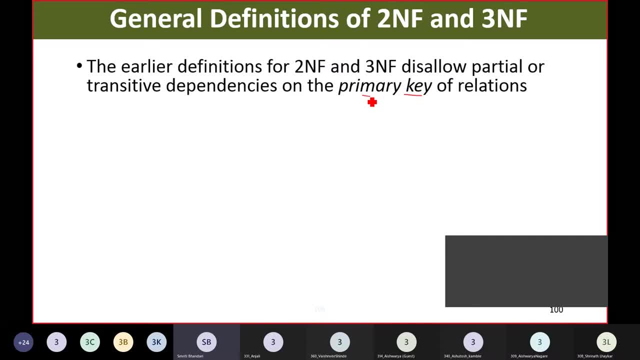 So in our definitions we said that no non-primary key attribute, no non-primary key attribute. So we considered only primary key right for partial or transitive dependencies. 2NF and 3NF are considered, But more general, if we would like to define 2NF and 3NF, we 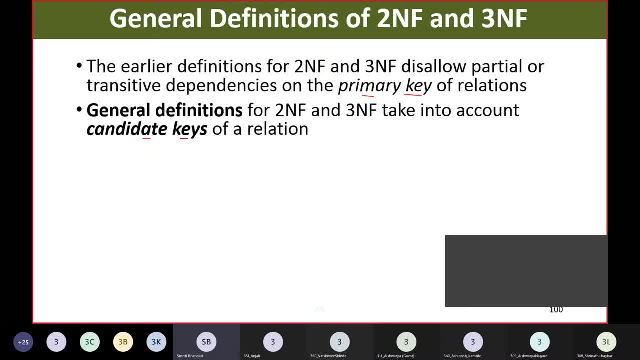 need to consider the candidate keys instead of only the primary key. We know the difference between the primary key and candidate key. For a relation, we may have more than one candidate keys and out of those candidate keys we designate one candidate key as the. 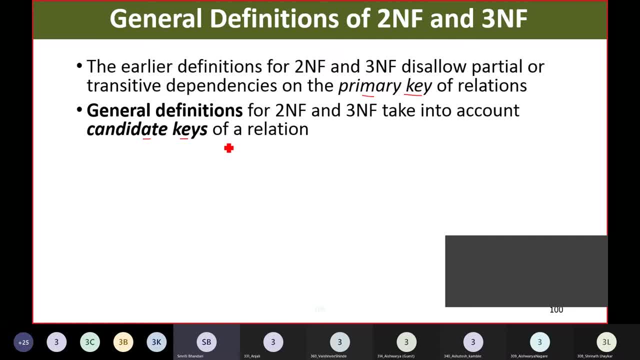 primary key that we know right. So so far in the definition we considered only the primary key, single one primary key of the relation, right. But if we would like to generalize those definitions of 2NF and 3NF instead of considering only the primary key, then we 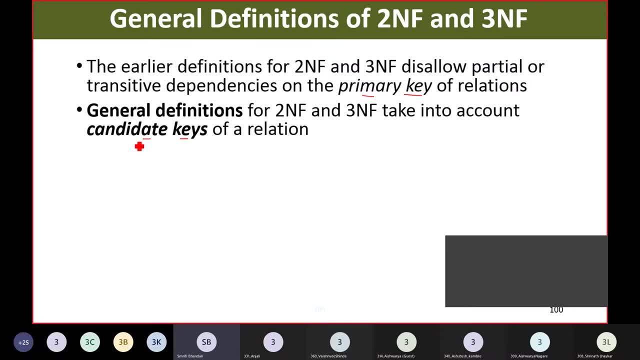 are considering the candidate keys of the relation. So the general definition of 2NF now becomes like this: A relation that is in first normal form and every non-candidate key. See here we are saying every non-candidate key. Earlier we were saying every non-candidate. 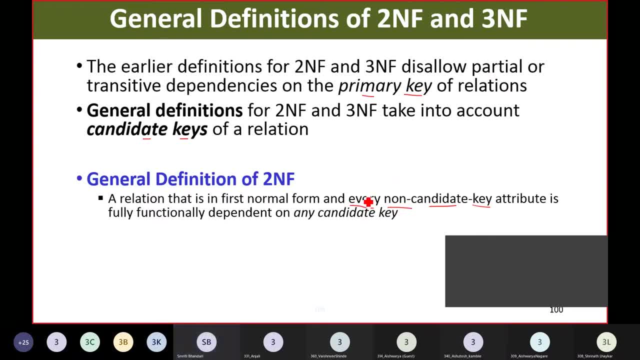 key. Now we are saying every non-candidate key. Now we are saying every non-candidate key and non-primary key, Every non-primary key attribute. That was the earlier definition. Now, while generalizing the definition of 2NF instead of considering a single primary, 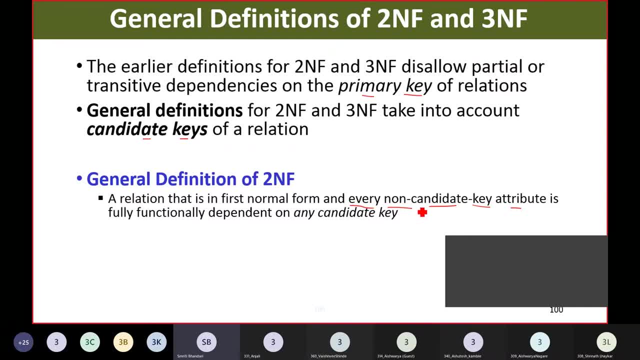 key. we are considering all candidate keys. So we are saying that a relation that is in first normal form and every non-candidate key attribute is fully non-candidate key. It is fully functionally dependent on any candidate key. So that is the difference. 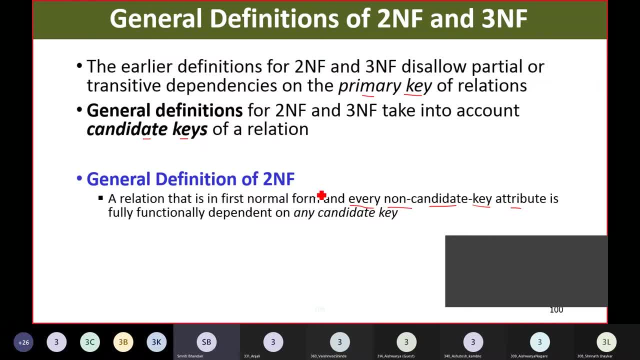 So obviously this form of 2NF, general definition of 2NF is somewhat complex than the earlier definition And it is putting more constraints. Similarly, if we go for general definition of 3NF, once again here also. 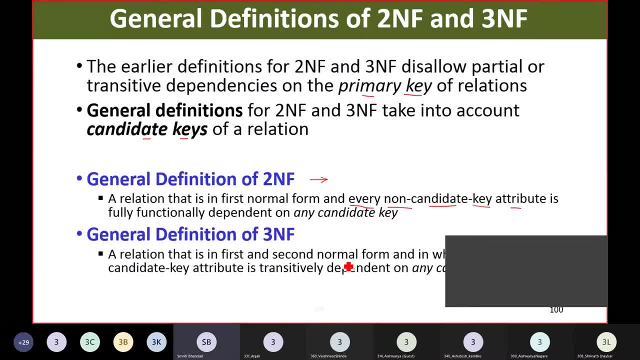 We say that a relation that is in first and second normal form and in which no non-candidate key attribute is transitively dependent on any candidate key. So here also we are not simply restricted to a single primary key, but we are more generally saying that no non-candidate 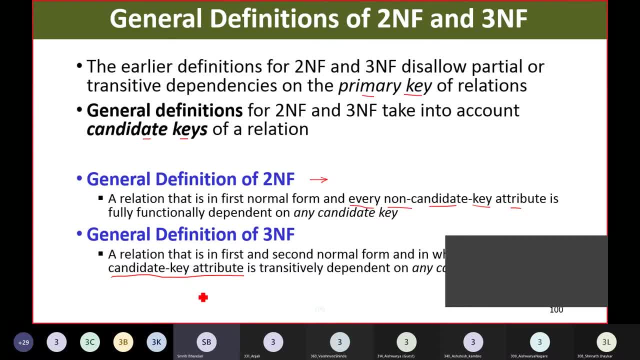 key attribute. So we may have more than one candidate key and we are generalizing the concept to all those candidate keys. So once again, this general definition of 3NF becomes more complex and it will put more constraints right. 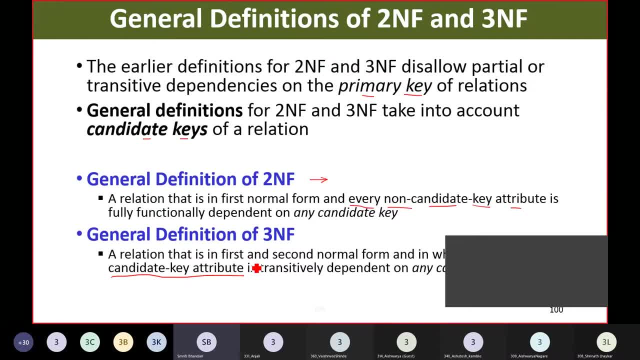 So I hope you must have understood the difference in general definition and the definitions, those we have discussed earlier, right. So these definitions actually put additional constraints on the relations And these definitions may identify few hidden redundancies in the relations right. 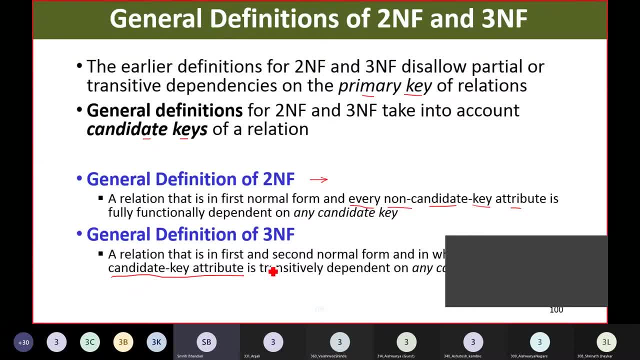 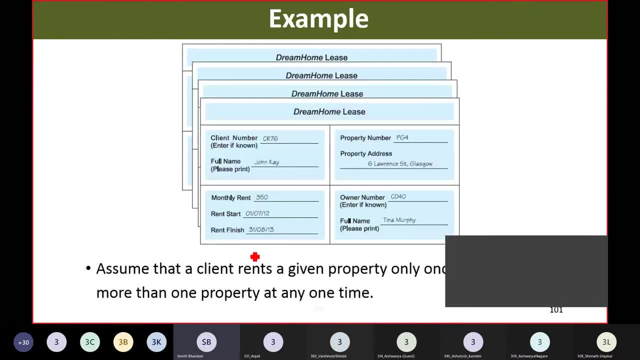 So obviously the process of normalization, if we use these definitions, would be more complex. okay, Fine. So let us proceed now once again with our. So let us proceed now once again with our example of dream house. So we have discussed. 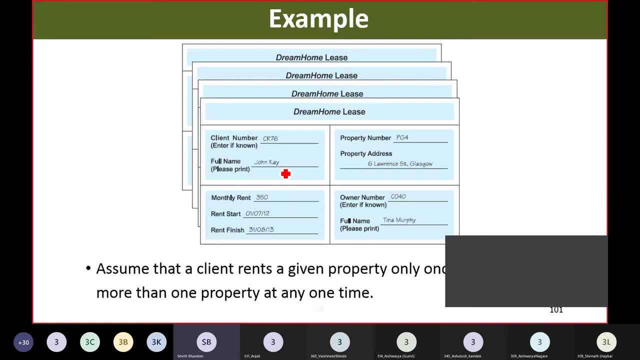 this example for discussing the earlier normal forms. those were 1NF, 2NF and 3NF. So once again we are referring to this dream house case study. Assuming client rents a given property only once and cannot rent more than one property at any one time, right? So we? 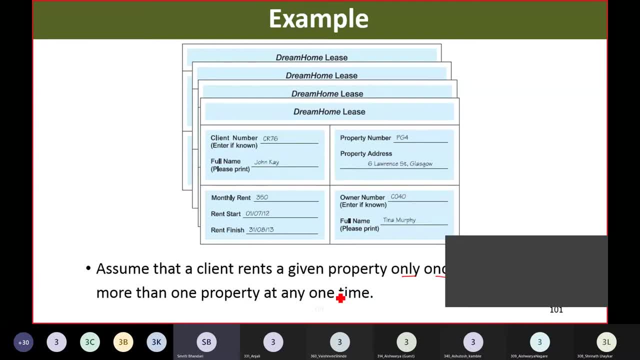 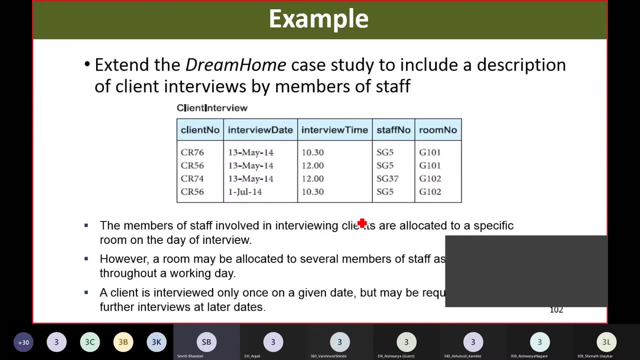 have seen this problem. We have seen this problem statement earlier and we have discussed 1NF, 2NF and 3NF for this problem. Okay, Now we are extending this dream home case study to include a description of client interviews. 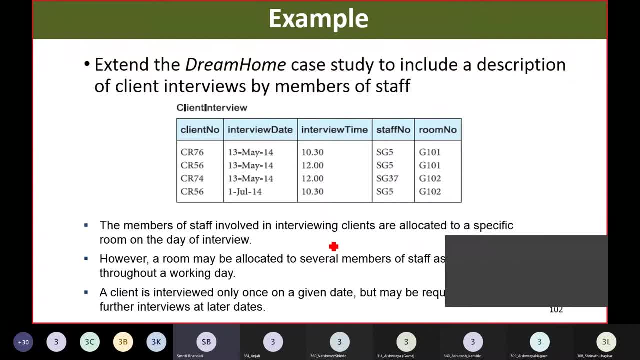 by members of staff. So now, apart from the earlier information that we stored in our dream home database, we would like to store some more information related to client interviews and what that information is. we want to store the information like the staff members are carrying out the interviews of the clients on a particular interview date and time. 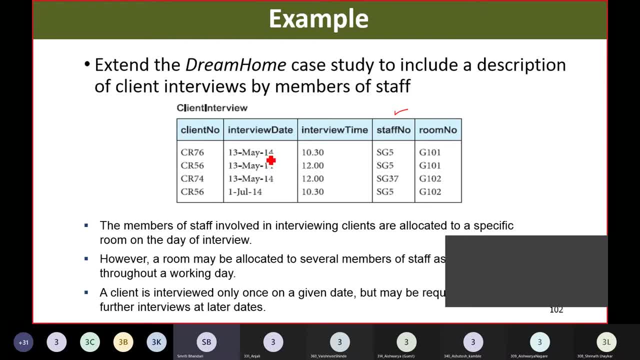 right, and these interviews are scheduled on those particular dates and times for the respective clients and to conduct those interviews, some room numbers are allocated, right, so we would like to store the information, like which client is having interview on what date, what is the time of the interview, who is this staffer? 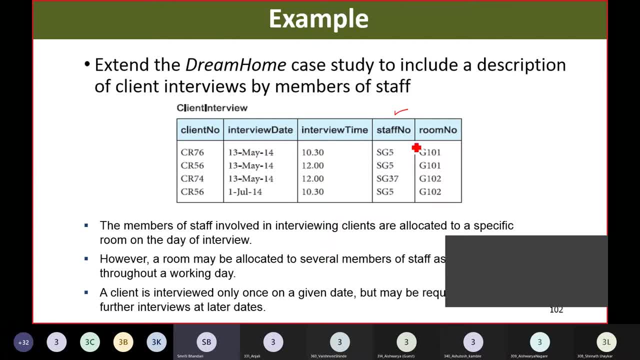 who is conducting that interview and what is the location for that interview. so this information, additionally, we would like to store in our dream home database system, right? so please see here few statements are being provided from which they extract some functional dependencies for this relation. so what is the information provided? let us go through. 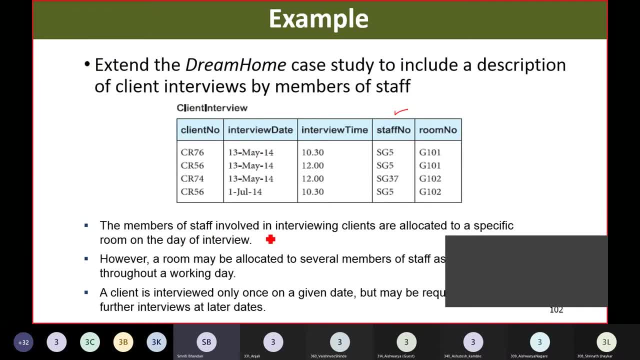 the members of staff involved in interviewing clients are allocated to a specific room on the day of interview. so staff members who are conducting the interviews on a particular date are allocated a specific room to conduct that interview. right, however, we are, tile at A room may be allocated to several members of staff as required throughout a working day. 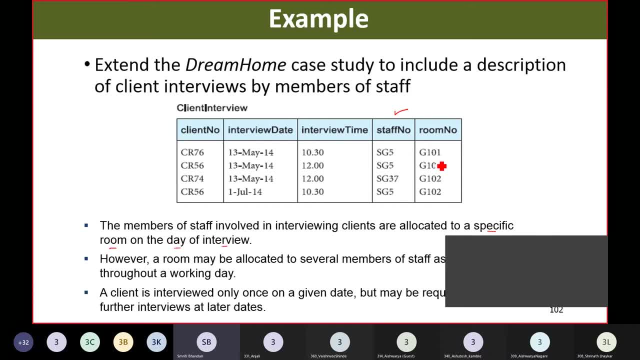 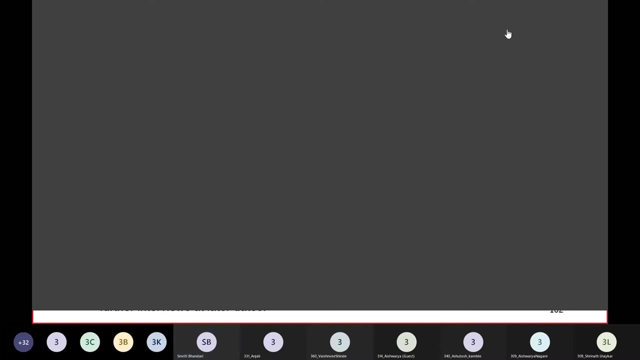 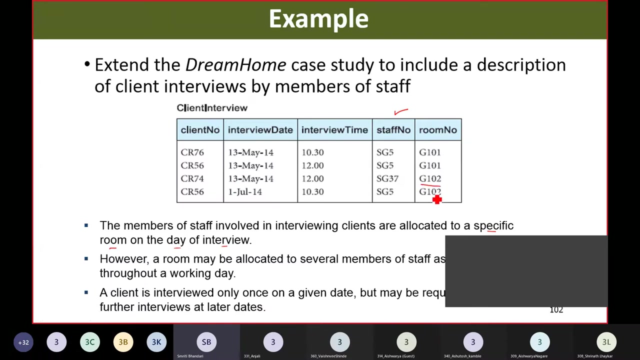 This means that not necessarily one room is allocated to one staff, But one room may be allocated to more than one staff. Say, for example, if we look at this information that we have, What we see here is: see here this room number G102, right. 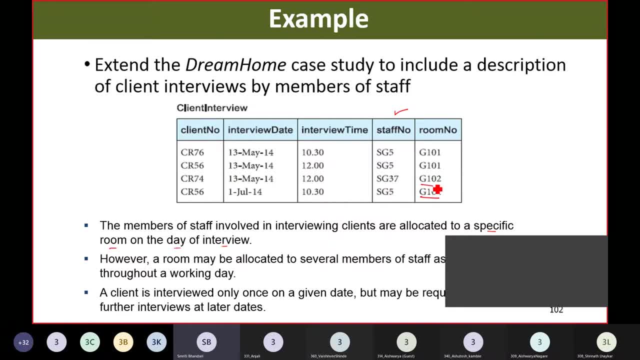 So this G102 is being allocated to two different staff members. Also, we can observe here that this staff number, SG5, is having three interviews scheduled right. So the interviews those are conducted on same date are at same location, But for the same staff number, SG5, the interview that is conducted. 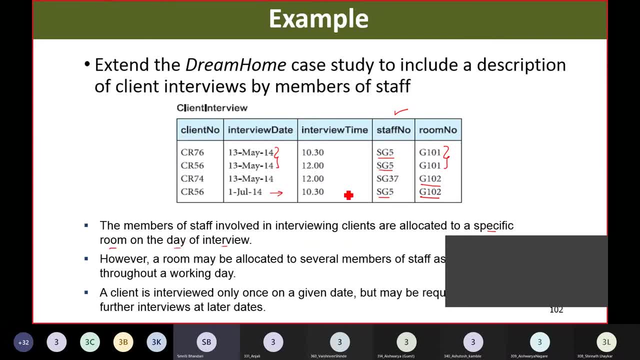 That is scheduled on different date is having different location right. So if we look at this data, we may come up with several functional dependencies. Further, it has been mentioned that a client is interviewed only once on a given date, But may be requested to attend. 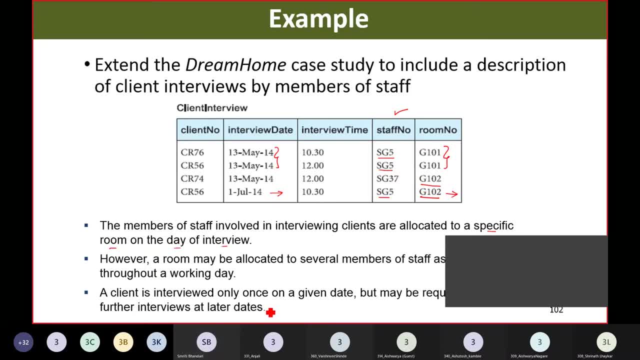 For interviews, right. What does this mean? See here: this is one client, CR56, on this particular date, 13th of May. This particular client will appear for interview only once on the given date, but for the same client it is possible that. 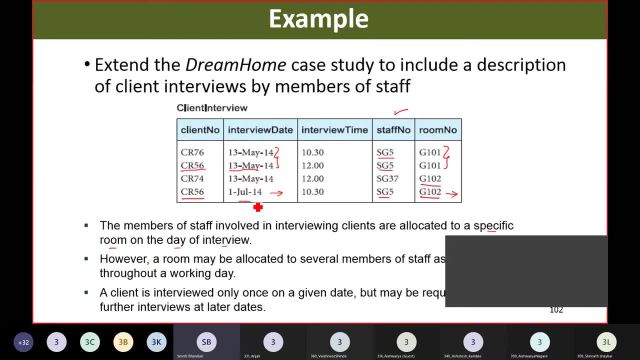 Few, Few more interviews are scheduled on different dates. So for the same client, CR56,, we are having one more interview scheduled here on 1st of July, right? So one client may appear for more than one interview on different dates. 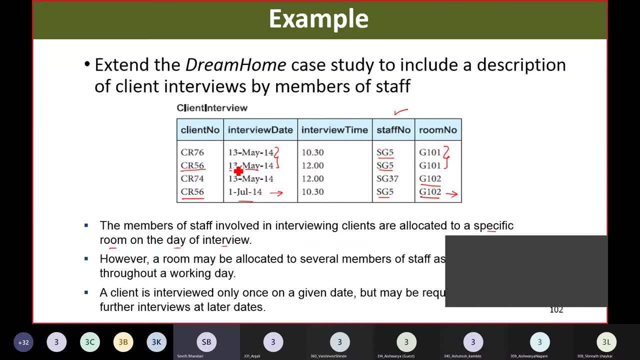 It will not happen that one client is appearing for the interview more than once on the same date. It will not be possible. Okay, so looking at the data, the description about the data that has been provided, we may come up with several functional dependencies, right? 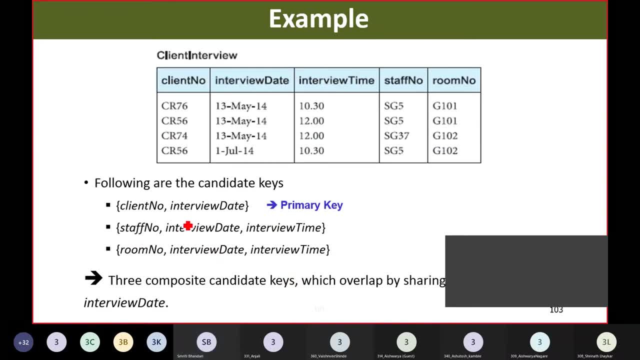 So what are the dependencies? Just look at it: We have identified few candidate keys based on the information that has been provided. So for this relation, we have identified that client number interview date would be our primary key. Client number interview date would be our primary key. 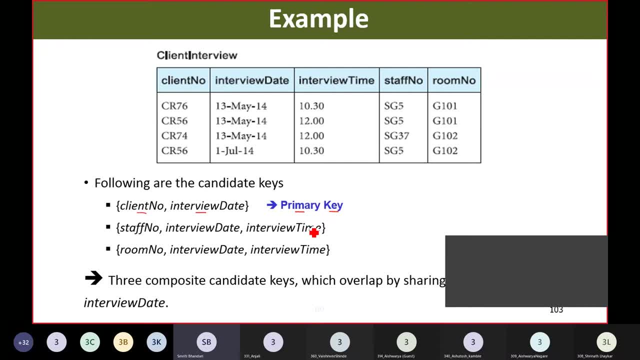 Further, we are having several other candidate keys as well for this relation. So what are those candidate keys? We have identified that staff number, interview date, Interview time would be candidate key. room number, interview date, interview time. that can also be our candidate key right. 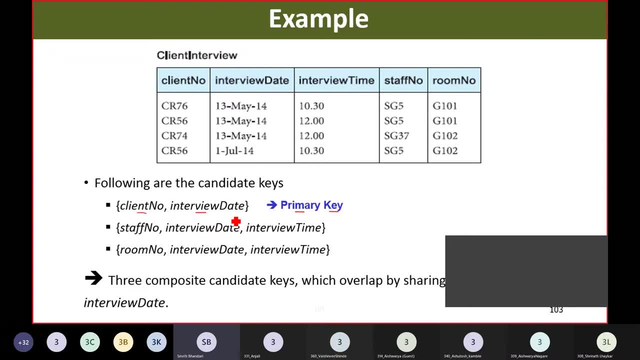 client number, interview date is also a candidate key and this candidate key is designated here as primary key right. so in a sense we have identified three different candidate keys, which are composite candidate keys, meaning the candidate key comprises of more than one attributes. every candidate key comprises of more than one attributes, and that is why we say that. 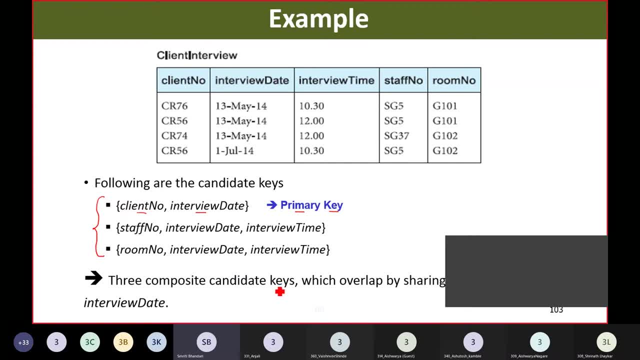 these com candidate keys are composite candidate keys but if we look at these candidate keys, these candidate keys are sharing one common attribute and that is interview date. so in every candidate key we are having this interview date common. that is just the observation right. are you getting me? 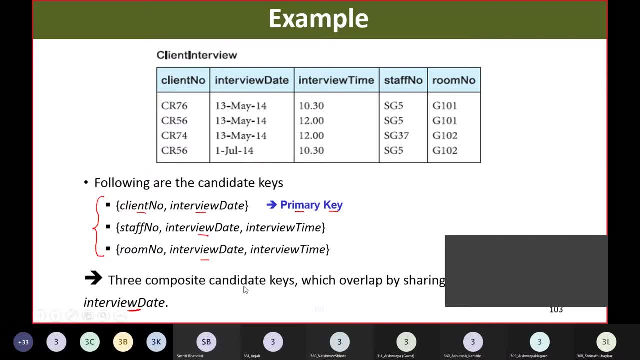 yes, also. yes, ma'am, see, please, if you have any doubts, please interrupt me and ask your doubts, right? so, these are very important concepts and that is why, in case, if you are not able to understand the concepts, please interrupt and ask your doubts, right? so let us proceed now. 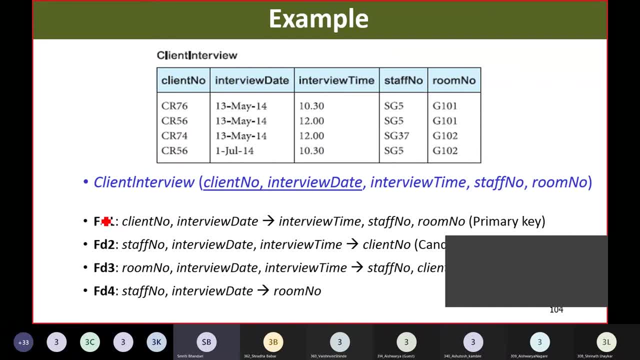 with our discussion. so, as i stated, we have identified three candidate candidate keys. one of the candidate keys is designated as the primary key right now. further, if we look at the information that has been given, we may come up with one more functional dependency and what that dependency is. 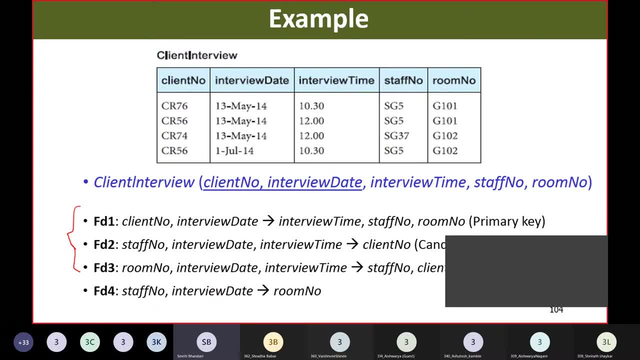 see here: staff number interview date determines room number. is the functional dependency that we are identifying here. what is the dependency? staff number interview date is determining room number. do you agree with me? is this the valid dependency that we may have, the сти that we may have? yes, 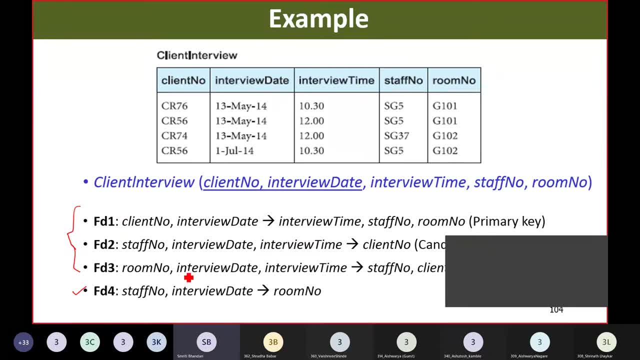 just look at this dependency. what we are saying: staff number, interview date determines room number. it is the staff numberProיס. what we are saying: the staff number of interview date determines room number. in fact, in our description we have been provided with one statement. the members of staff involved in analyzing and enjoying the statements. 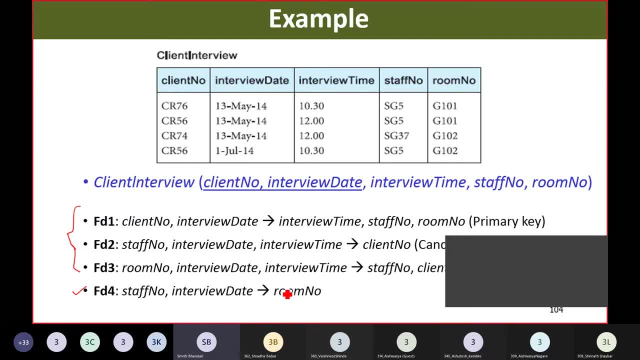 number group imitate the number of members of staff involved in analyzing or considering of the counseling process. interviewing clients are allocated to a specific room on the day of interview. so for a specific staff, on a specific date, a specific room number is been allocated. that is the statement is given as, like this, the members of staff involved in interviewing clients. 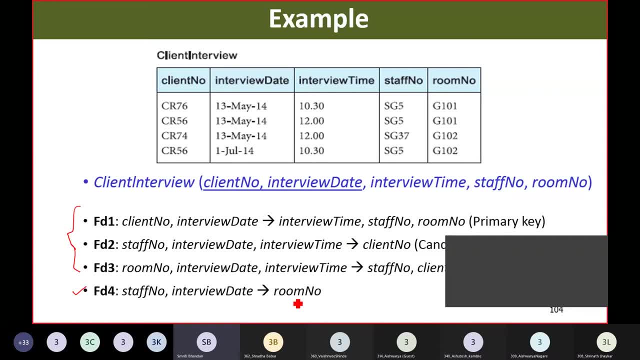 are allocated to a specific room on the day of interview, right. so specific staff number on a specific date has been allocated with a specific room number, right. and that is why we are having a functional dependency like this. we are not saying that staff number determines room number. 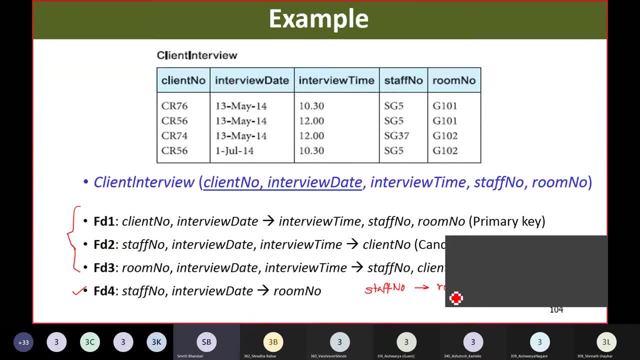 is this the valid dependency? staff number determines room number. see here. staff number sg5. room number g101. staff number sg5. room number g101. but for the same staff, sg5, we are having here another room number, g102. staff number will not determine room number. 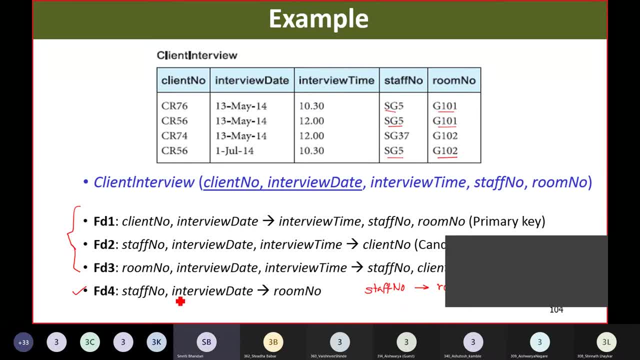 so this is not valid. but staff number on a particular date: staff number on a particular date, right will be allocated a specific room. so staff number, interview date- will determine room number, because on a particular date the same staff number is allocated, the same room number got it and that is how we have come up with this functional dependency. 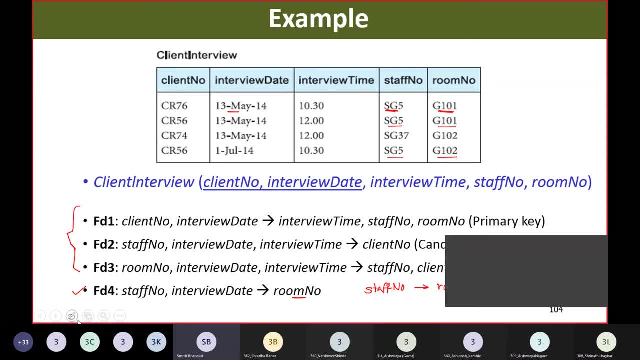 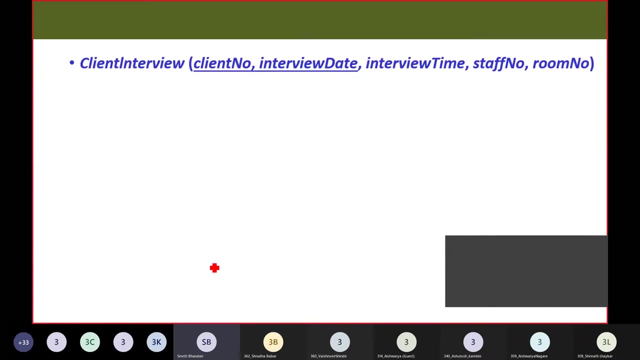 are you getting me? yes, yes, are you so clear with this dependency- staff number, interview date, determining room number, please? fine, so let's proceed now. this is our relation. we have identified primary key as client number, interview date, right, so we want to know whether this relation is in 3nf. 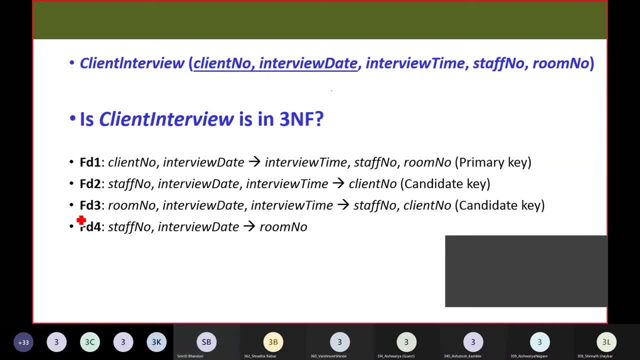 we have identified these dependencies right. so what we want to know is whether this relation- client interview- is in third normal form. whatever third normal form says, what is the definition? it should be in 1nf and 2nf. so our relation is in one nf and 2nf, no doubt. and the second 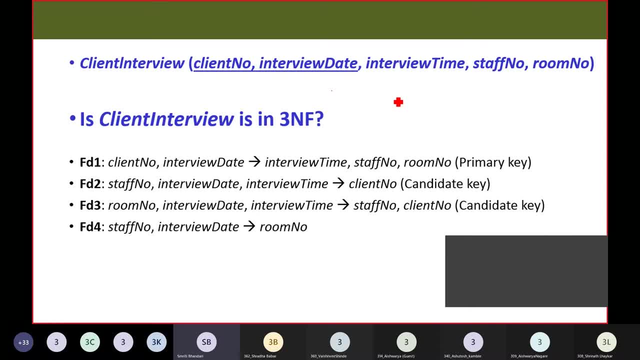 condition says that every non-primary key attribute, every non-primary key attribute, should not be transitively dependent on primary key right. so, if we look at this dependency, no problem with these functional dependencies- fd1, 2 and 3, because all are my candidate keys. so no issues with these dependencies right. one more important point you may. 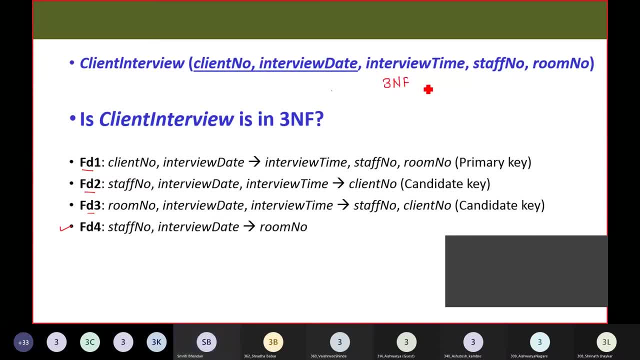 consider, while discussing 3lf, that if we are talking about a functional dependency of the form alpha to beta, right, and if this is my candidate key or this is my super key right, if all the dependencies are having the determinant as super key right, then we need not consider those dependencies. definitely the relation would be in 3lf. 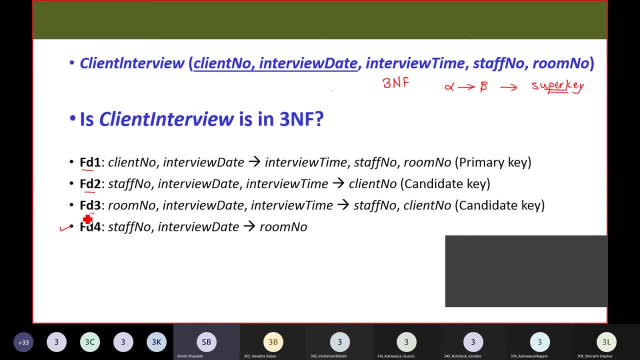 okay. so if we are talking about these first three dependencies, these are the candidate keys. so always if the dependency is a candidate key for the relation, there will not be any problem. problem to declare the relation whether it is in 3nf or not. it is always in 3nf. but in addition to these, 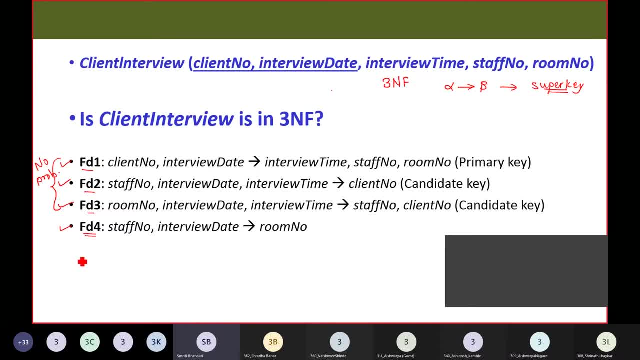 dependencies. we are having one more right, so we need to think of, or we need to pay attention to this dependency and we need to check whether this dependency is violating our rule of 3ll. So if we look at this dependency- staff number, interview date, determining room number- right- then obviously we may say that there is no transitive dependency. this is not the transitive dependency as such. 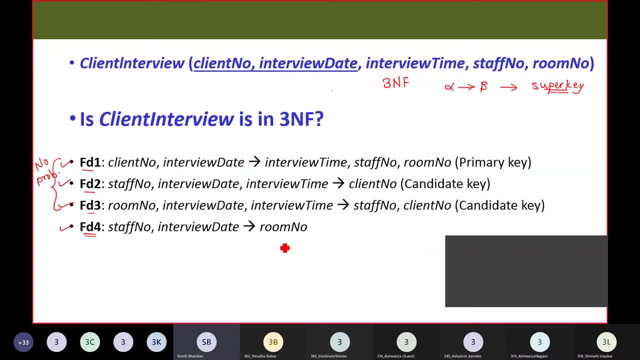 So if we come up with a transitive dependency on the primary key or in general, on the candidate key, then we may say that the relation is not in 3LF but here. whichever functional dependency we are looking at, this is not the transitive dependency. 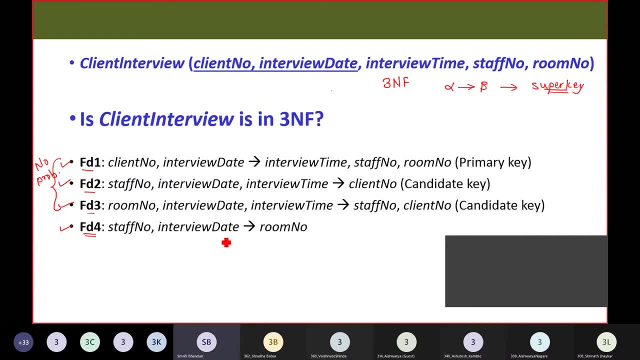 Right. so, even though this staff number, interview date is not a candidate Key for the relation, this functional dependency is allowed in 3LF right, because room number, which is the right hand side of the dependency, is part of one of the candidate keys. This right hand side room number of this dependency is part of one of the candidate keys and this is allowed. 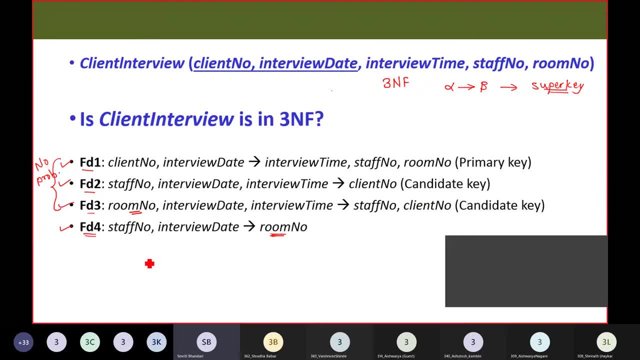 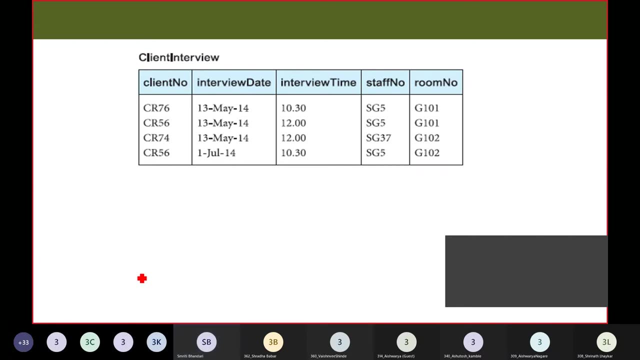 In 3LF. right, and that is why we may say that this relation is in 3LF no issues. okay, but now, if we look at this particular relation, Whether this relation suffers from any kind of update anomaly- Yes, whether this relation suffers from any kind of update anomaly. 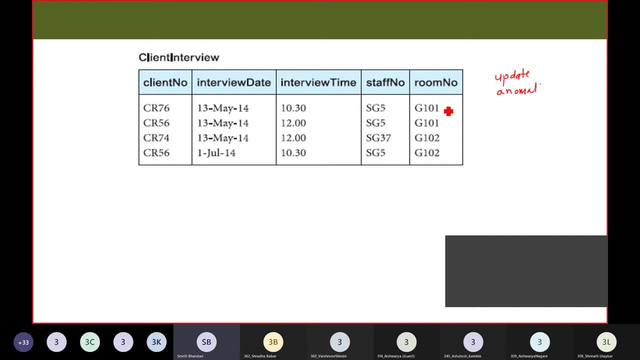 Or, in other words, I may pose a question like whether there is any kind of redundancy. Yes, Yes, Yes. Is there any kind of redundancy exist in this relation? I am expecting the answer from you people. We declared that this relation is in 3LF. 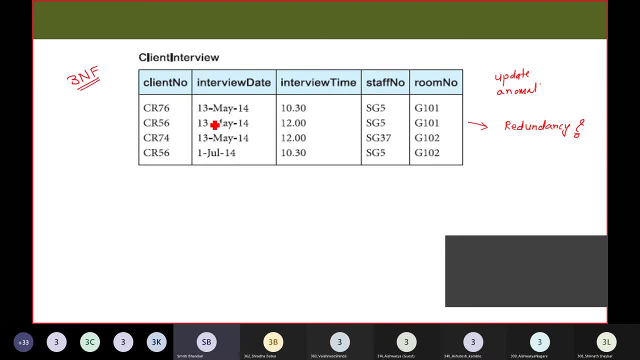 No doubt, Okay, But But if we look at now this relation, whether there is any kind of update, anomalies, or in other words, if whether there is any kind of redundancy present in this relation. Yes, Yes, If we look at this instance, 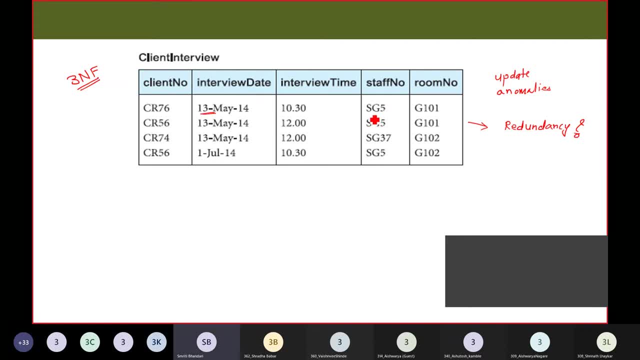 On date 13th of May, this staff number, staff number SG5, is allocated this room G101, right and on the same date for same staff number. in this particular relation we are having two entries right, So it may happen that one staff is conducting. 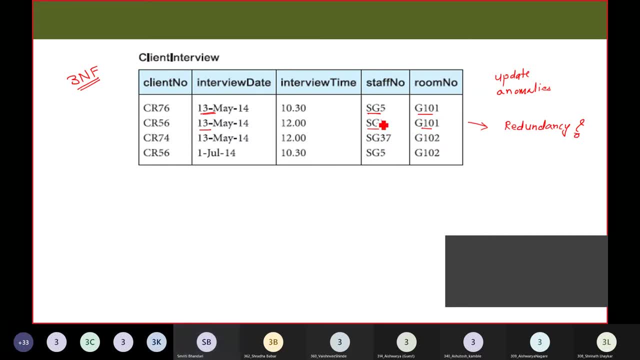 Several interviews Of different clients on same date. Do you agree with me? Yes, Are you getting me or not? Yes, ma'am, So So. So, meaning If The same staff Is conducting More than one interviews on the same date. 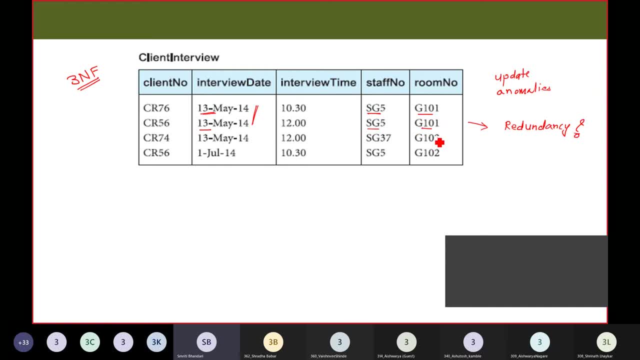 Right, obviously that staff is allocated the same room number. So if for this particular staff, if I'm having ten entries on same date because this staff member is conducting ten interviews, Let us assume- Then this room number will be repeated for 10 times. 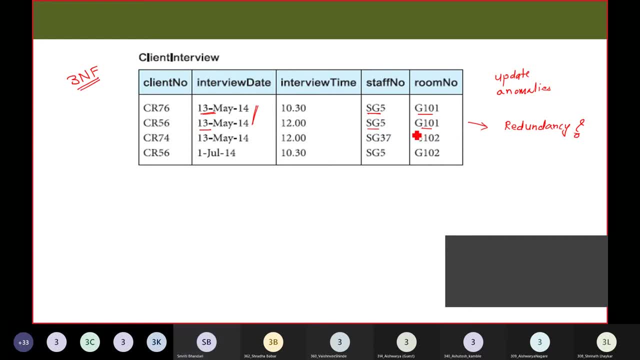 Is that correct Here? in this instance the room number is repeated twice because this staff number SG5, on 13th of May has allocated room number G101 and this staff is conducting two interviews on that date, right? So the same room number is repeated twice here. 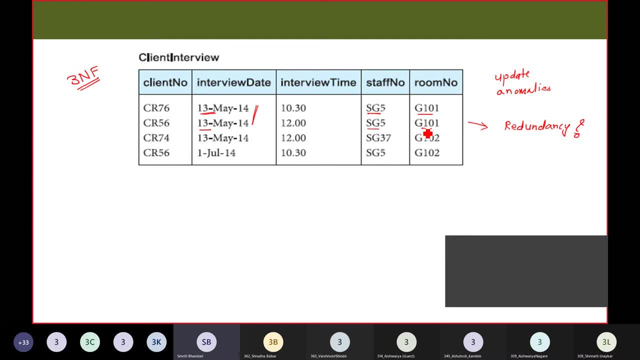 So if, by some reason, if it happens that the room number allocated to SG5 needs to change due to some reason, then obviously if the room number allocated earlier to this SG5, if that room number needs to be changed, then obviously all the tuppers. 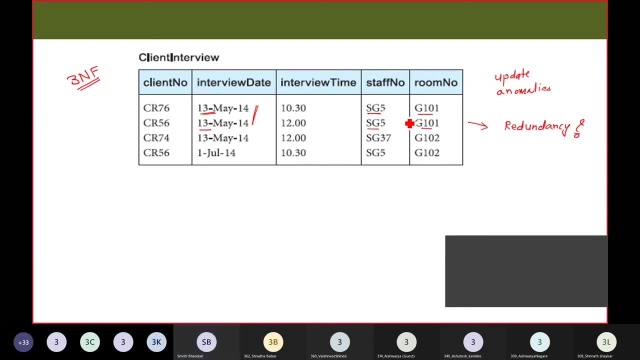 All the tuppers need to be updated. So here say, for example, for this staff, SG5, on 13th May: earlier this staff on this day was allocated with G101, but now, due to some reason, that room number needs to be changed. 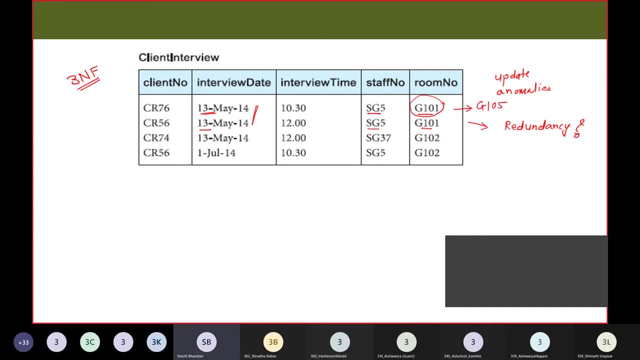 Two, So say, for example, G105.. So in this case, what we need to do is, as in this particular instance we are having two tuppers, we need to modify these two tuppers such that room number is now G105. 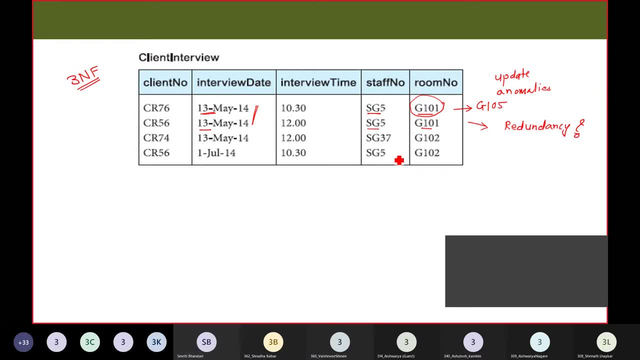 Are you getting me? Yes? Yes, And that is why we are saying that this relation suffers from update anomalies, meaning there is still some redundant data. So if we forget to change the room number for one of the tuppers, then it may happen that our data becomes inconsistent, right? 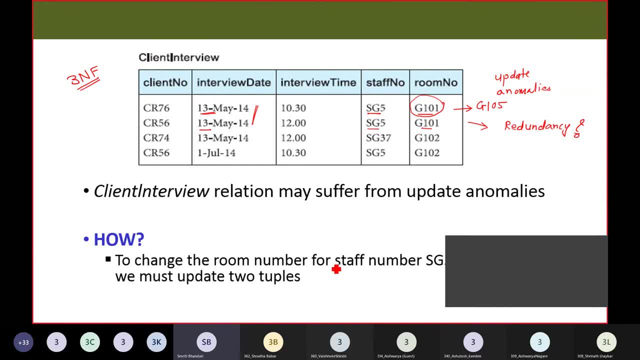 So why we are saying that there is update anomaly, Because to change the room number for staff number SG5 on 13th of May 14, we must update two tuppers with respect to this instance. Right, So what I want to convey is, though, this relation is in 3 and a third normal form. 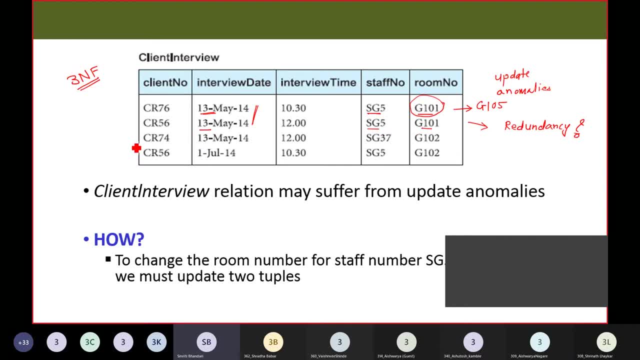 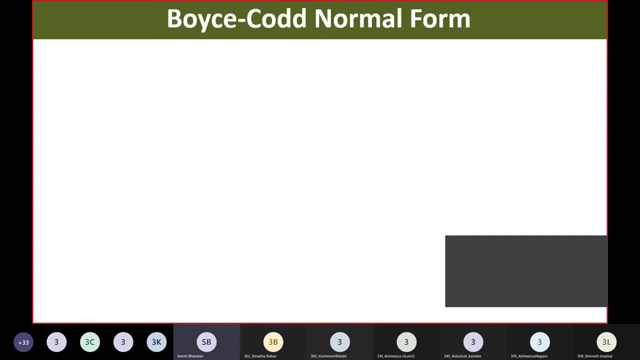 right. Yes, Yes, It may suffer from update anomalies. So even though the relation is in third normal form, we may have some redundancies still present, Right. So if we want to reduce or if we want to remove those redundancies in 3NF, we need to go for still higher normal form. 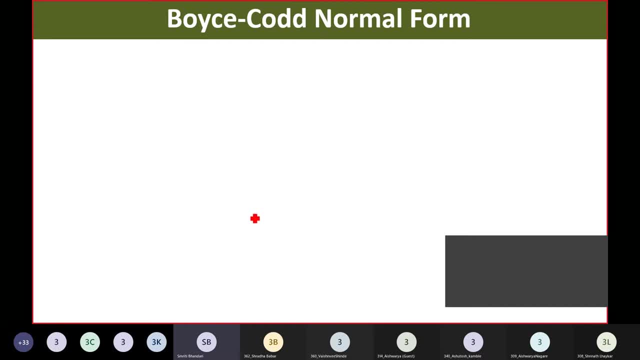 So if we want to reduce or if we want to remove those redundancies in 3NF, we need to go for still higher normal form, And that is known as Boyce-Codd normal form, or it is abbreviated as BCNF. This normal form was introduced by two scientists and those were Boyce and Codd and that is why the name BCNF- Boyce-Codd normal form. 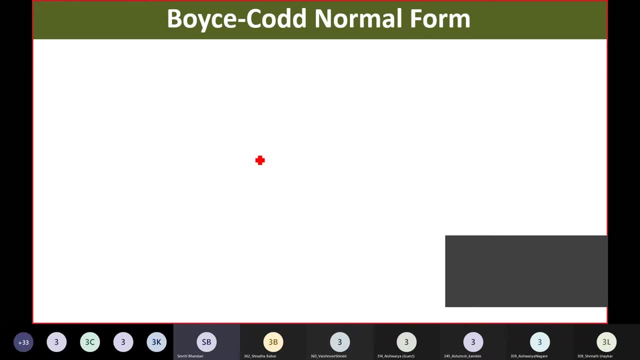 So to remove the redundancy that may exist. So to remove the redundancy that may exist in third normal form, we are coming up with still stringent normal form than 3NF, and that is known as BCNF. So let us try to define BCNF. 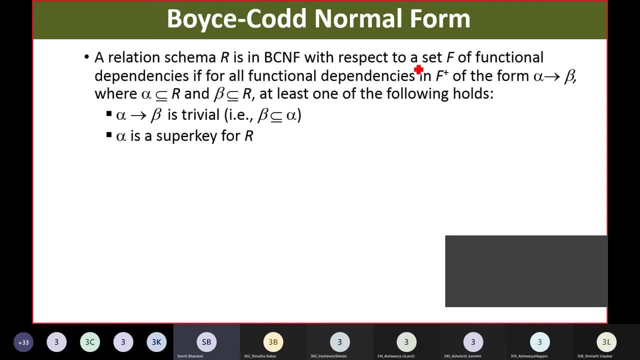 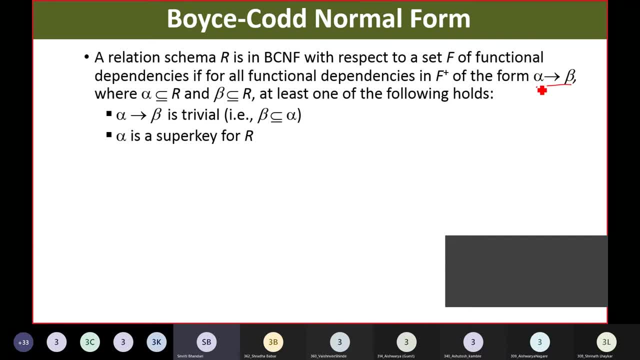 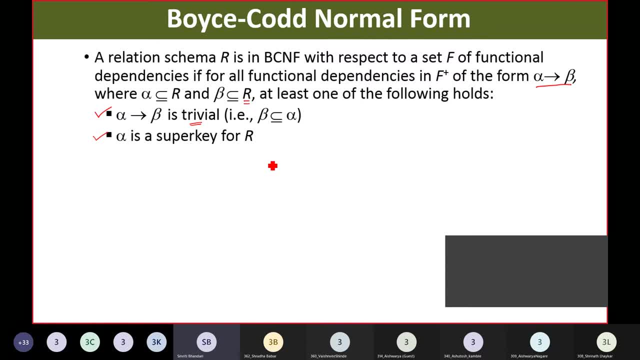 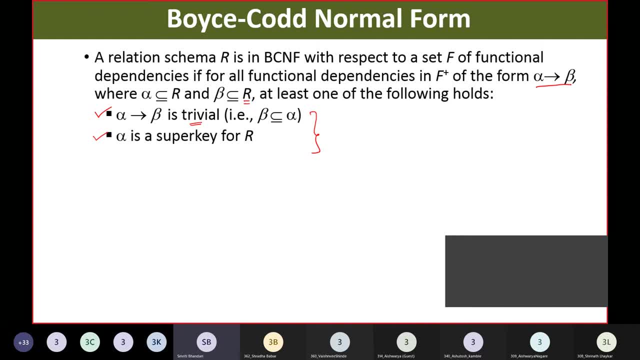 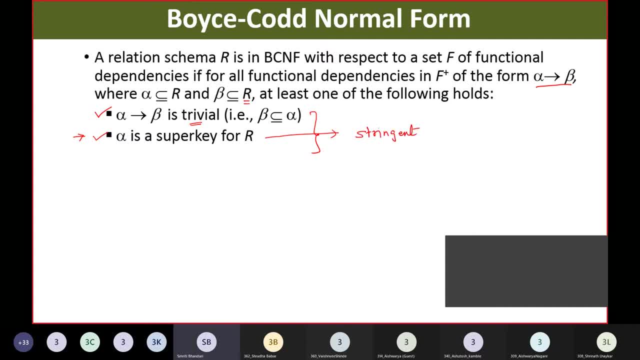 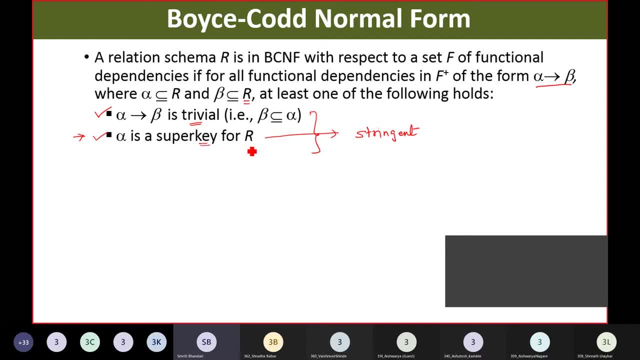 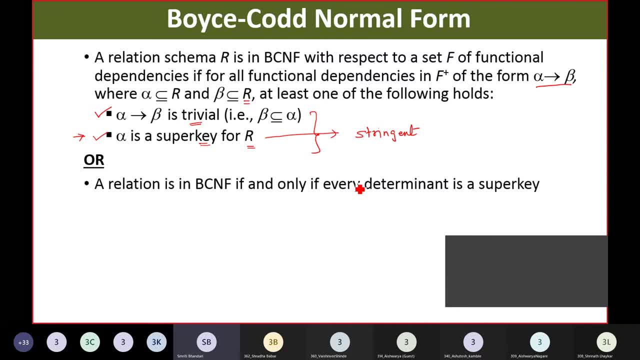 okay, so in other words, we may write this definition as: a relation is in bcnf if, and only if, every determinant is a super key. in simple words, we may say that further: the entire database design is in bcnf if each member of the set of relation schemas. 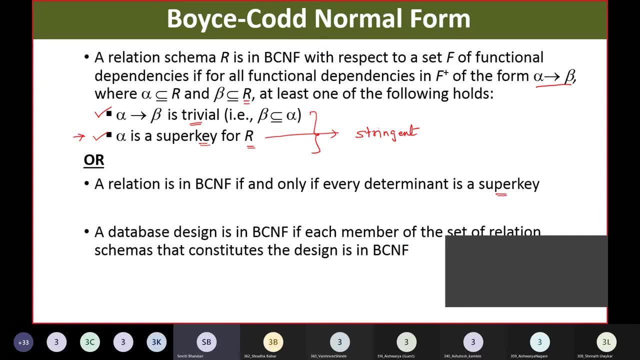 comprising this database design is in bcnf. so if i am talking about my university database, say for example, right, and if i am having several relations r1, r2 up to rn in this schema, then when i will say that my university database is in bcnf, 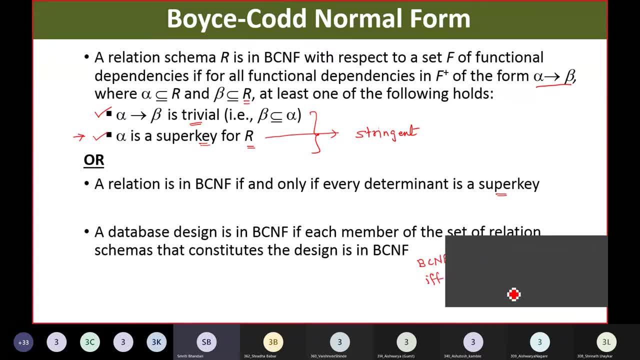 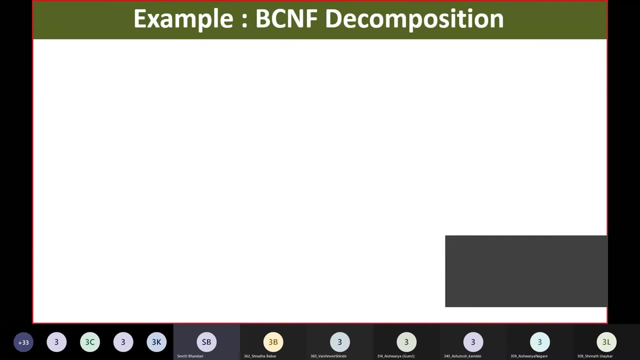 if, If and only if, every relation in this university schema is in BCNF, then and then only, I will say that the entire schema is in BCNF right Now. I hope you must have understood the definition of BCNF, which is more stringent than 3NF. 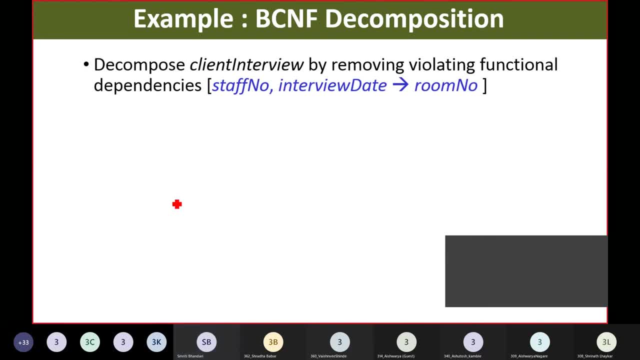 okay, Now let us see the example of BCNF. So, as we have seen, our client-interview relation is having this dependency- staff number, interview date, determining room number- right. So we said that this dependency is allowed in 3NF and that is why we declared that client-interview. 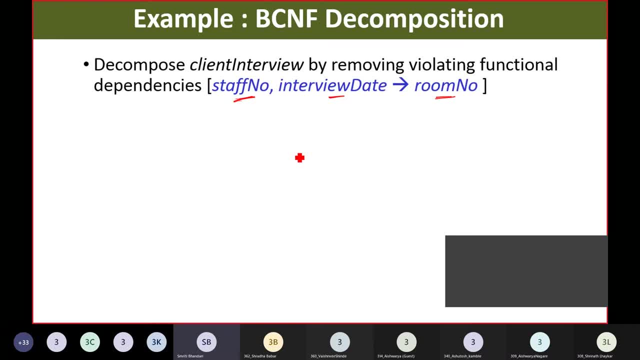 relation. So we have to check that the client-interview relation is in 3NF right, But due to this dependency, we are having some redundant data in our 3NF relation. So what we need to do is we need to check for this dependency. 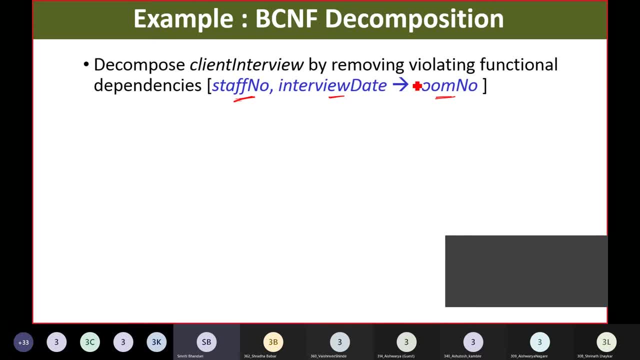 So if we look at this dependency, then whether this dependency satisfies the client-interview relation or not, whether this dependency satisfies the rule of BCNF, whether this dependency satisfies the rule of BCNF, what our rule says, if I am having a dependency of this, 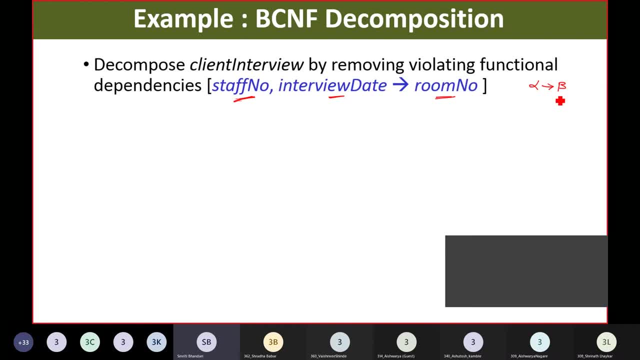 form alpha to beta either. this dependency is trivial. So first rule: this should be trivial dependency. What we mean by trivial dependency, Beta must be subset of alpha. So whether this condition is true in case of this dependency, This is my alpha and this is my beta, right? 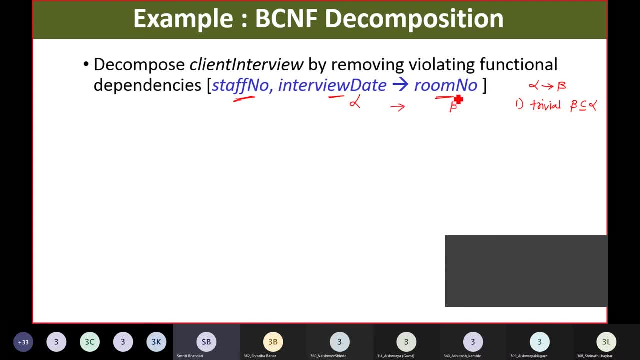 So whether this dependency is trivial, whether beta is subset of alpha, No, ma'am No, No. Therefore, the first condition is not satisfied, right? So let us check the second condition of BCNF. We are talking about BCNF conditions. 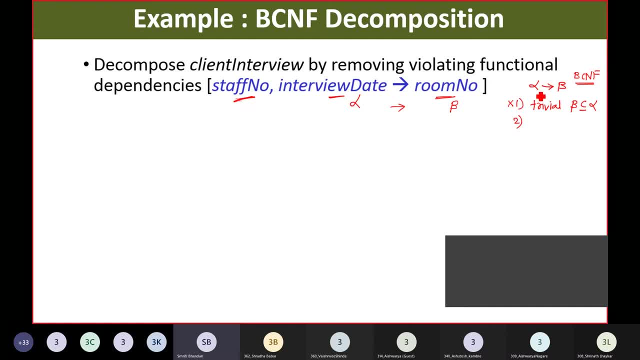 So what is the second condition of BCNF? In case of dependency alpha to beta, if the first is not satisfied, the second must be satisfied, And if the second gets satisfied, then only we will say That the relation is in BCNF. 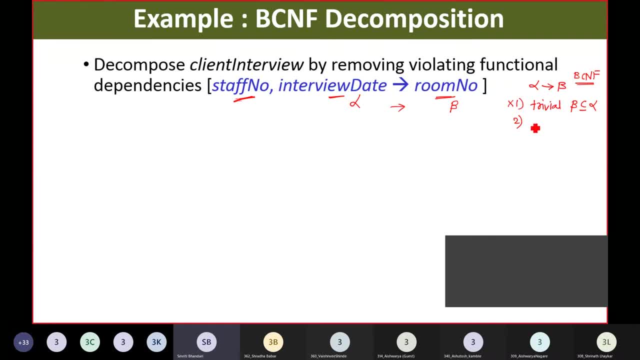 Otherwise no. So the second condition says that my determinant, that means my LHS, that means my alpha, must be the super key of the relation. So if I look at this staff number interview date of this functional dependency, staff number interview date. 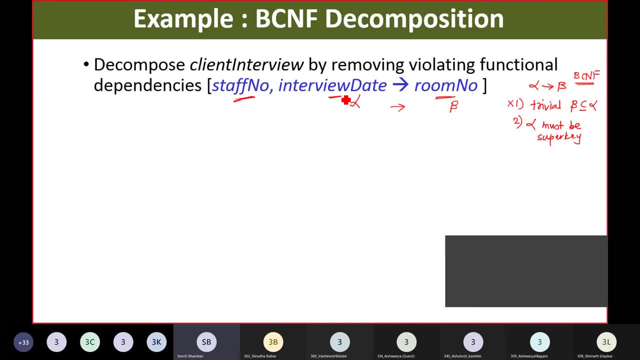 So if I look at this staff number interview date of this functional dependency, staff number interview date, Whether the staff number interview date determines all other attributes of the relation, Then, and then only, we will say that this is my super key. But if we look at our instance of the relation, then we may come across the situation where 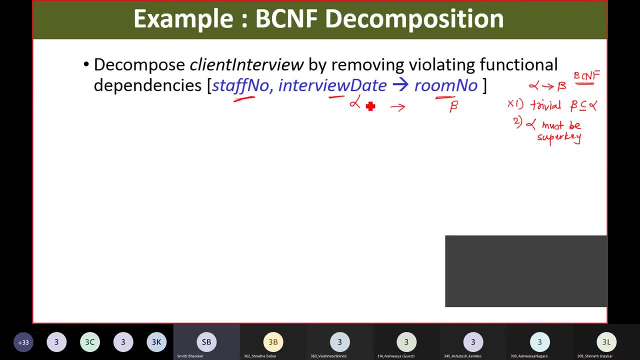 staff number interview date is not satisfied. So if I look at this staff number interview date, I will know that the staff number interview date is not satisfied, not determining all the attributes of this relation, and that is why staff number interview date is not my super key. so this second condition is also violated, right, and that is why we say that. 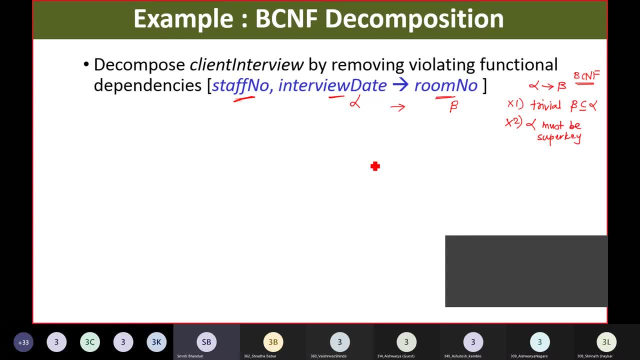 even though my relation client interview is in 3nf, it is not in bcnf. it is not satisfying the norms for bcnf boys called normal form. so what to do to convert our client interview relation in bcnf? what we need to do is we need to remove such kinds of functional 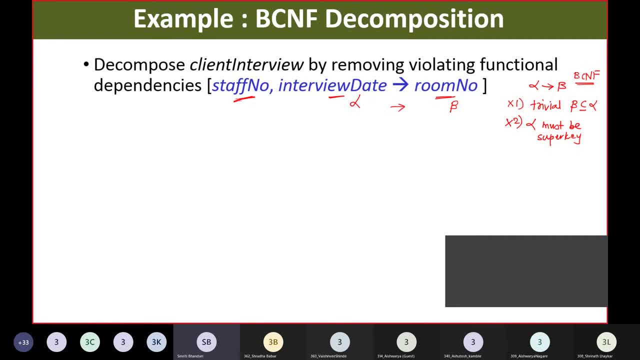 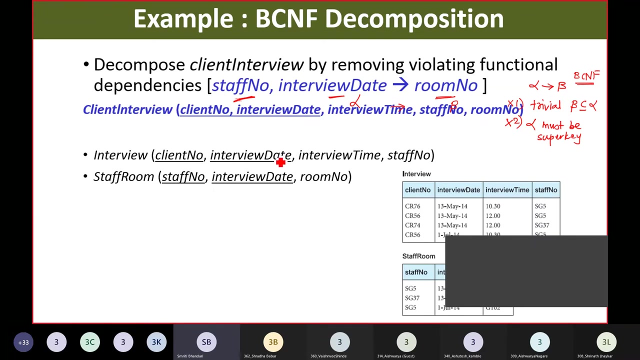 dependencies, those are violated under bcnf. so we need to decompose client interview relation now by removing this functional dependency which is violating my bclf rule right. so we are having this relation- client interview- so what we are going to do is to decompose. we are going to decompose our relation by making use of this dependency. 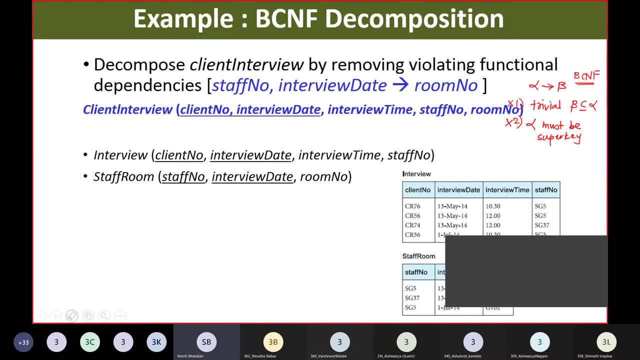 that we have identified which is violating the norm of bcnf. okay, so simply, we are applying the rule for decomposition, so we are having this functional dependency that is violating the rule. so, simply, while decomposing, we are going to make use of this work as a function of b chega function. 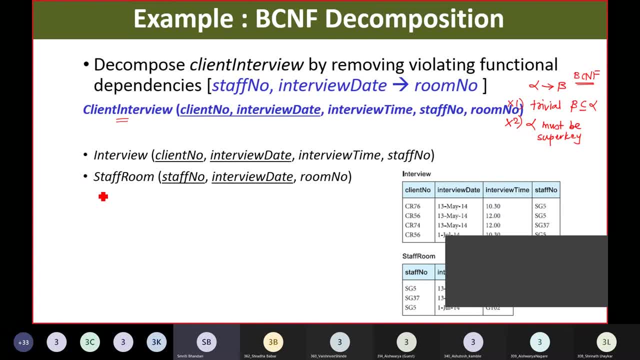 so, once we have all the functions, we will be decomposing this relation. what we will do is we will make use of these attributes in this functional dependency and we will come up with a separate relation. see here: staff room, having staff number, interview date and room number- three attributes: okay, so we have done. 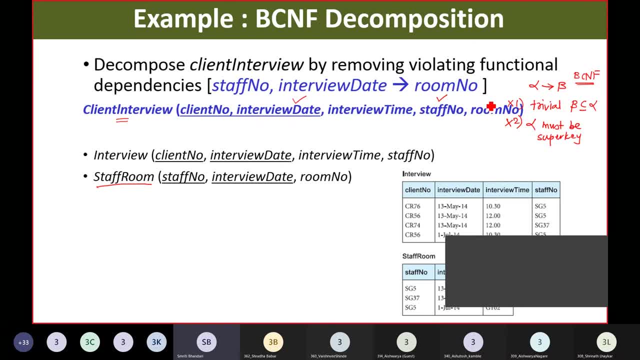 with staff number, interview date and room number. okay. now whichever are the remaining attributes? say, for example, this: client number, interview time- those are remaining attributes, okay. so what we need to do is we need to come up with the another relation wherein we are having this remaining attribute- client number, interview time also, we need to have this primary key of 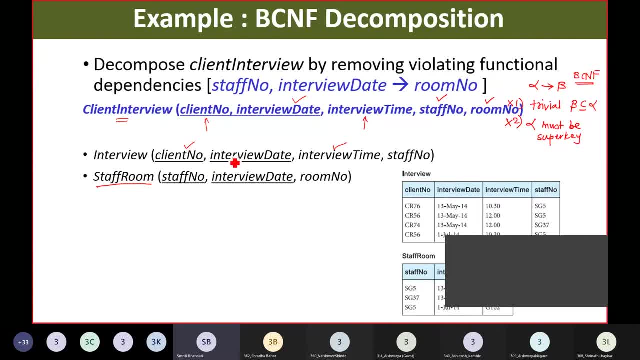 staff room relation. that should be included in my interview relation. okay, so staff number- interview date- should be included in my interview relation. okay, so staff number- interview date should be included, also be present in this interview relation. so my interview relation will have four attributes: client number, interview date, interview time and staff number. so now after. 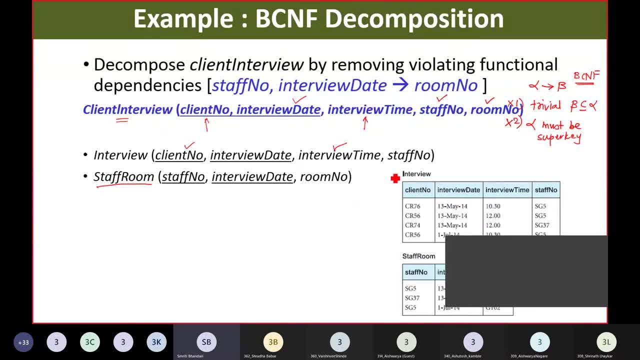 decomposition. our client interview relation is decomposed into interview and staff room. interview relation will have four attributes and staff room will have four attributes. for this case, shame if you have Conversationaczego untuk Re spel. Terzi novo tiredismo- three attributes. Is that correct? So earlier, what was the redundancy in client-interview? 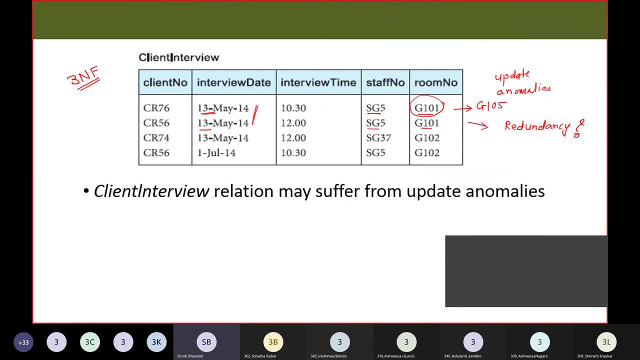 relation. Let us go back In client-interview relation. we had the redundancy- And what was the redundancy? If on the same date the same person is having more than one interview scheduled, then room number was repeated Correct And that was the redundancy in 3NF. 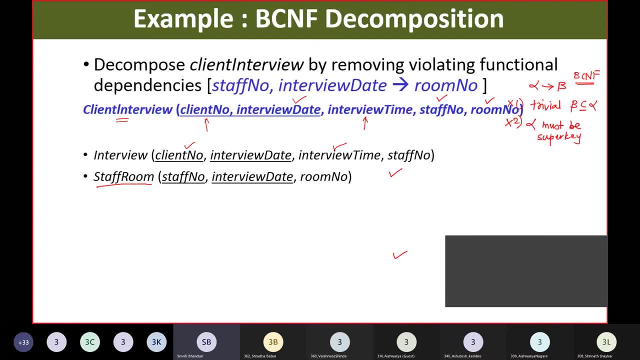 So what we have done now is we have converted this relation in BCNF by making use of this dependency- staff number, interview date, determining room number- Right- And we have come up with this separate relation- Staff room- Wherein we are having staff number, interview date and room number. 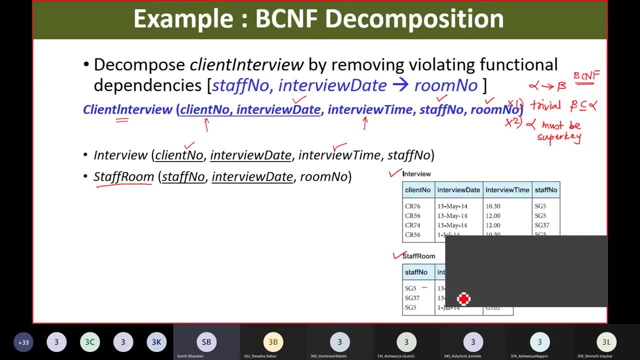 So for a particular staff number on particular interview date, this room is being allocated. So if we would like to change the room number for a particular staff on particular date, we need to update only one entry, Because there is no redundant entries. now, Correct. 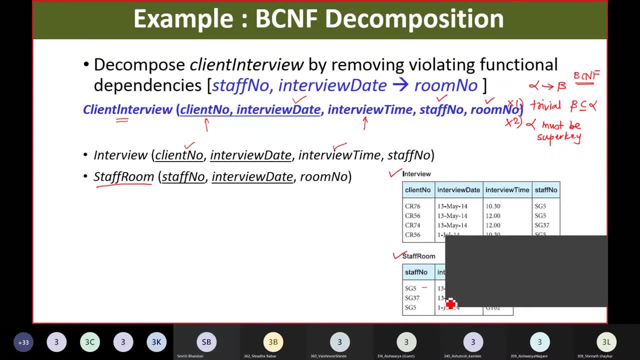 on the same date for same staff number, right. So only once we need to modify this room number If it happens that the room number is changed In earlier case, whenever our relation was in 3NF, due to the schema of 3NF and due to this functional dependency. 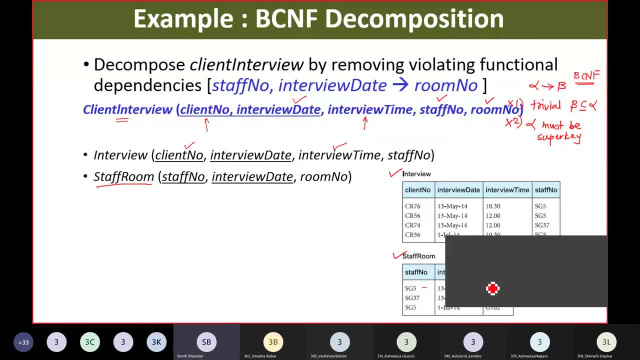 we have to change more than once the room number If it happens that the room number is changed on a particular date for a particular staff, right. But now we have decomposed the relation and we have removed the redundancy. So it is possible for us now to remove the redundancy in 3NF. 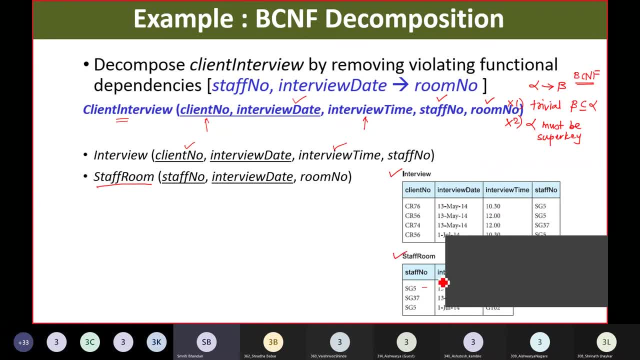 And we have come up with now this BCNF decomposition right, And that is why we said that BCNF is more stringent than 3NF, because it is not allowing any redundancy. now, okay, But BCNF is not always variable. BCNF is not always desirable. 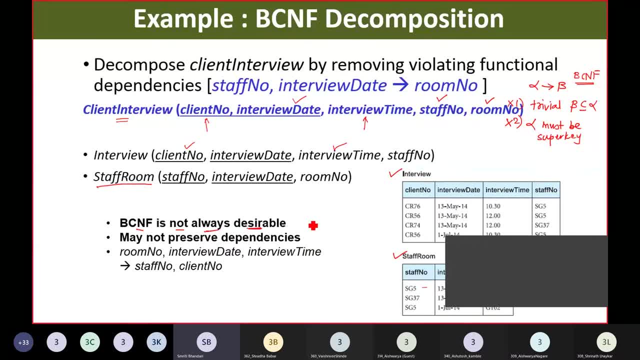 Why? What is the reason why I am saying BCNF is not always desirable? No doubt, if I am having the relations in BCNF, I will not be having any redundancy, But there is a problem. There is a problem in BCNF sometimes. 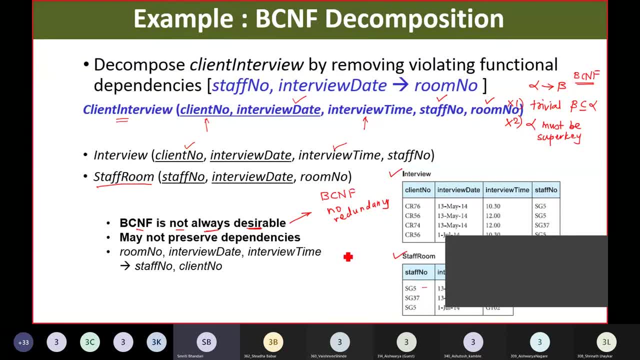 And what is that problem In BCNF? it may happen that few of the dependencies are not preserved, So BCNF may not preserve the dependencies. What we mean by dependency preservation? We have A discussion at length regarding this dependency preservation right. 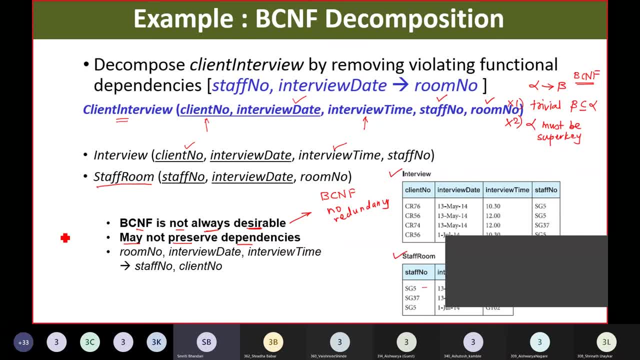 So, in simple words, what we mean by dependency preservation: If I am having a dependency and if, to check for that dependency, if I need to compute join of two relations, then I will say that that dependency is not being preserved And without computing the join of two relations. 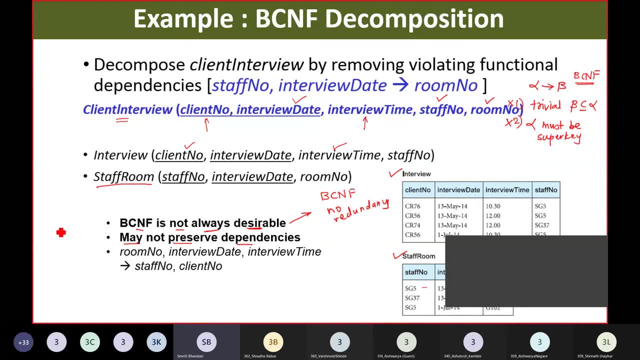 if I am able to check for the functional dependency, then I will say that my dependency is preserved After decomposition. Now if we look at this dependency room number and set it as two number- interview date, interview time, determining staff number, client number- We are having 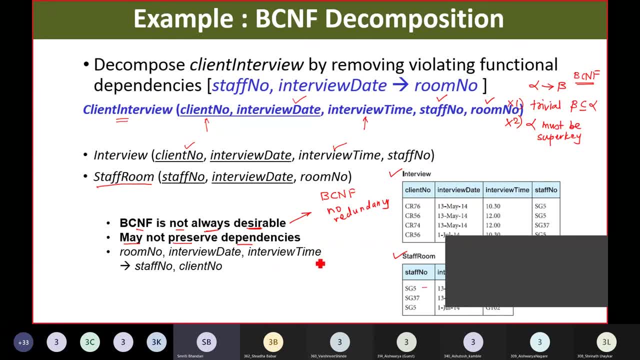 this dependency: Room number, interview date, interview time- determining staff number, client number. Right Now, if we want to check for this dependency, this is our decomposition, BCNF decomposition- And if I want to test for this dependency then if I look at the 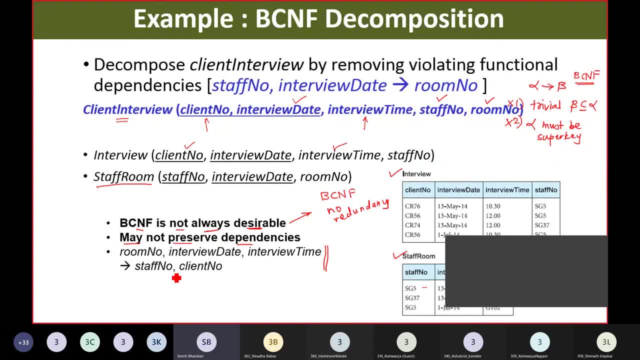 attributes in this relation. right Then, the staff number is present in this relation as well as this relation, But this client number is present in this relation only. Room number: interview date- interview time. Room number- interview date, interview time. 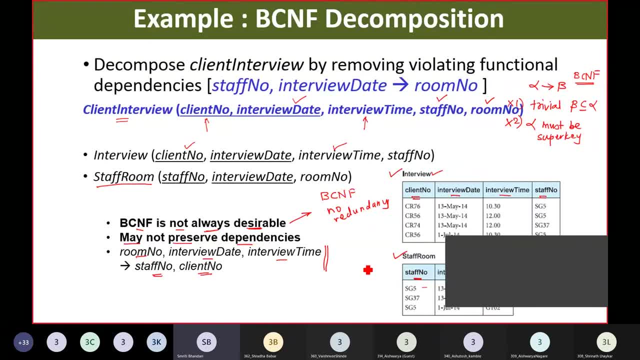 So interview date and interview time are present in interview. But if I want to check for this dependency in left-hand side, I also want room number. Room number is not available in the same relation. So to test for this dependency, I am going to check for this dependency, I am going to. 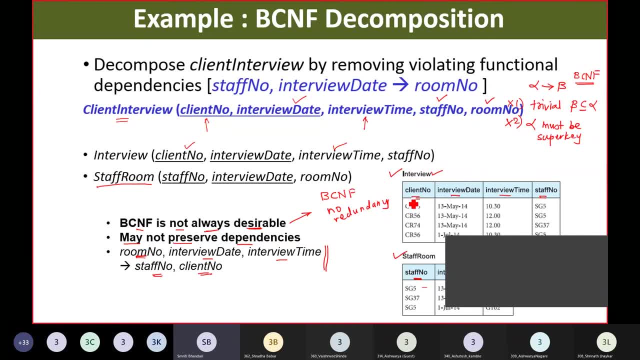 check for this dependency. What I need? I need to find the join of these two relations, because room number is available in staff room- Okay- And client number is available in interview. So if we look at all those attributes in the left-hand side- few of the attributes- 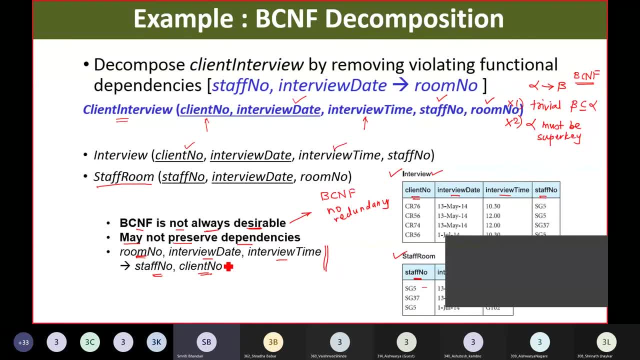 are present in one relation. So if we look at all those attributes in the left-hand side, few of the attributes are present in one relation. So if we look at all those attributes in the right-hand side, few of the attributes are present in other relation. and if this is the 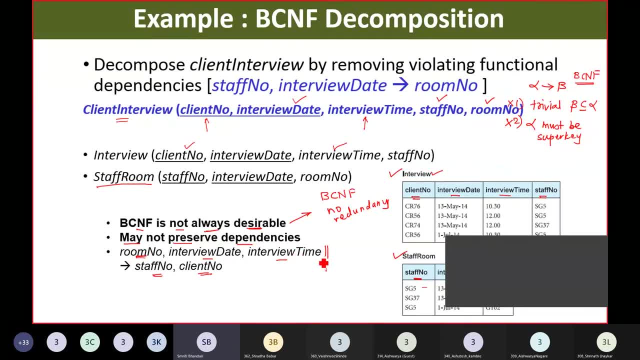 case, then we say that this dependency is not preserved. This dependency is not preserved, Right. So the disadvantage of BCNF is that sometimes it may happen that few of the dependencies are not preserved, and to check for those dependencies then we need to compute the 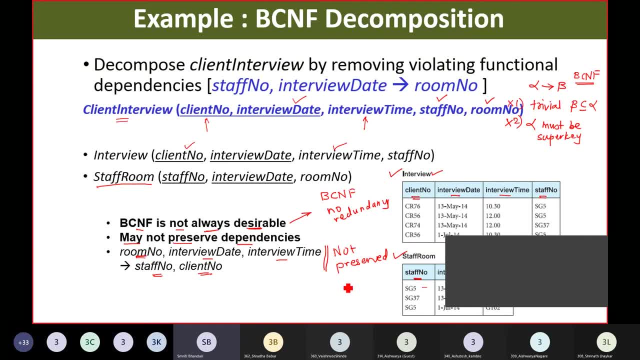 joints, and while computing the joints we may incur some overhead, right? so the advantage of bcnf is there is no redundancy, and the disadvantage of bcnf is sometimes the functional dependencies are not preserved, right? so if we are having two normal forms, those are, 3nf and bcnf, then we should think of, or we should have a wise decision. 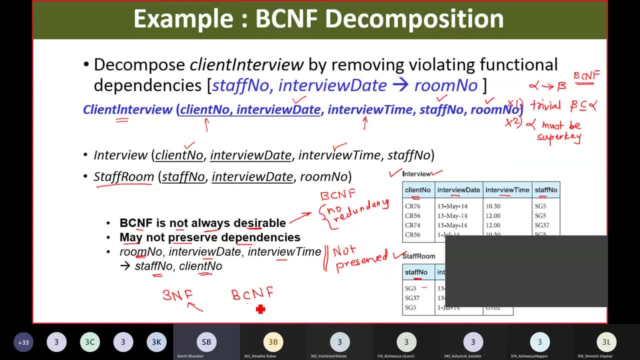 which normal form to be used, whether we should go with 3nf or whether we should go with bcnf. obviously bcnf is more stringent than 3nf, meaning bcnf will not allow any kind of redundancy. so if we are more concerned about the redundant data, then obviously we should go for bcnf. 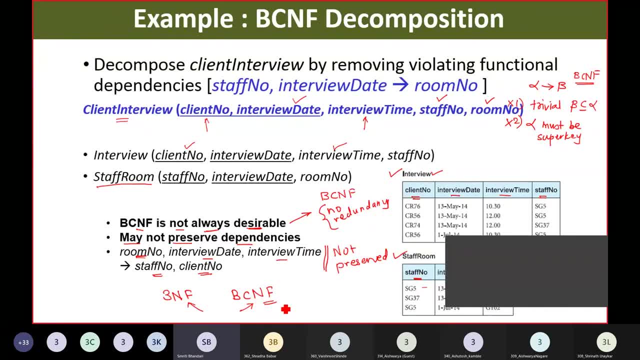 but if we are more concerned about testing the functional dependencies, then obviously we should go for bcnf and we should go for 3nf. And if there exists the dependencies those are not being preserved in BCNF, then we should stick to 3NF, right. 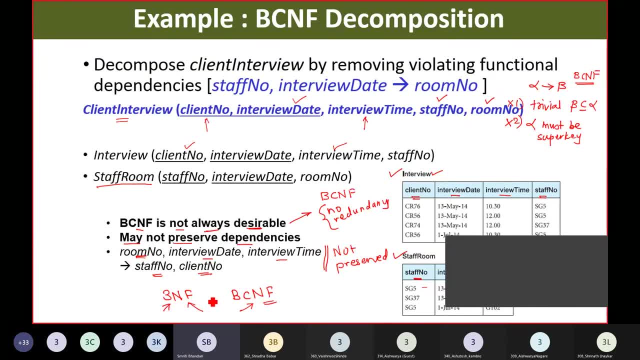 So, while designing a database, we should always think of this trade-off, whether we are more concerned about redundancy or whether we are more concerned about preserving the dependencies. So, in brief, I may say that 3NF will always preserve dependencies, right. 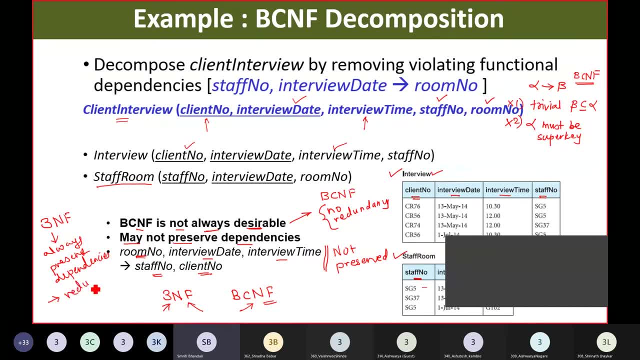 But the drawback of 3NF is we may have redundancies. We may have redundancies in 3NF. okay, If we look at BCNF, then BCNF will not have any redundancies. but sometimes it may happen that there are certain dependencies those are not being preserved, right? 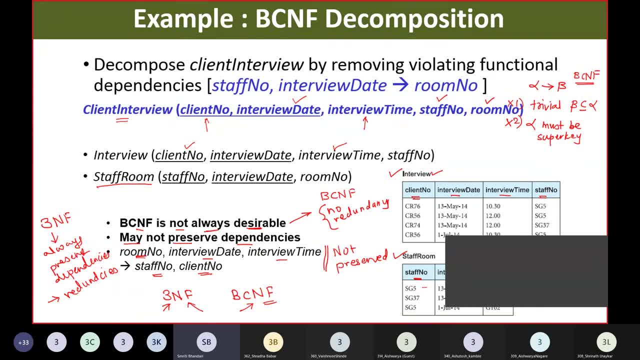 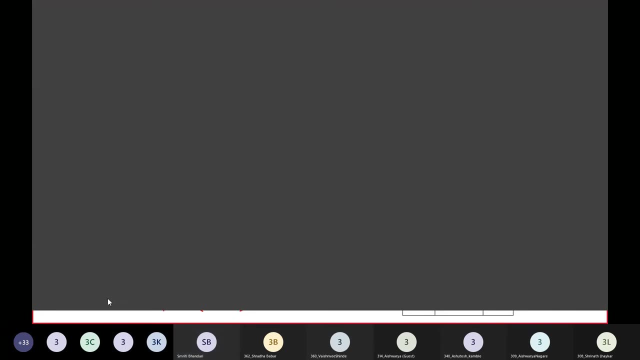 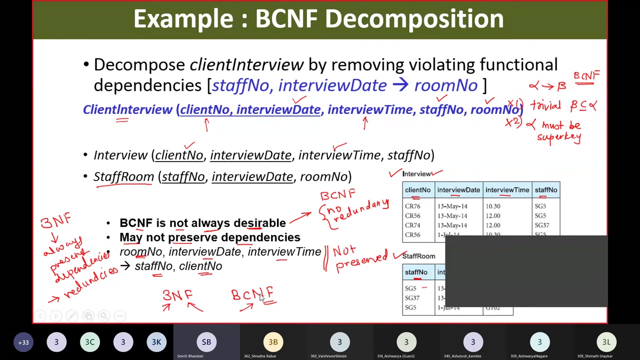 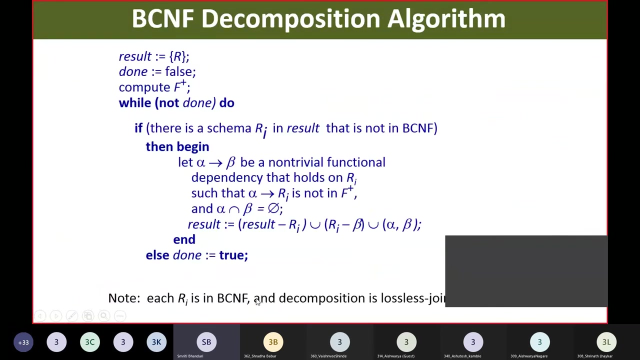 And that is why we should have a wise decision Whenever. Whenever we select one of these two normal forms, 3NF or BCNF, right? If you have any doubts, please let me know. Yes, Is there any doubt? So let me proceed with a formal algorithm for BCNF decomposition. 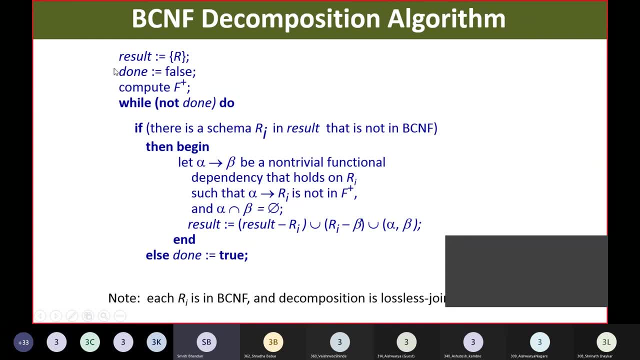 So we are having here a formal algorithm for BCNF decomposition. So let me go through this algorithm. In fact I have given you the trick how to decompose the relation In 3NF, In 3NF into BCNF, right. 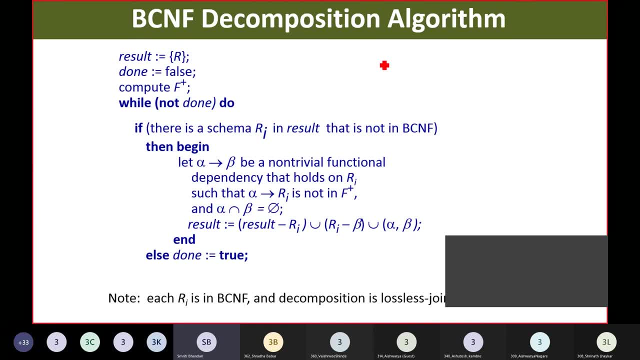 So, simply, we need to pick the functional dependency that is violating the norm of BCNF. And whichever is the functional dependency that violates the norm of BCNF, that functional dependency is being used to decompose the relation. The same thing is being mentioned in this algorithm formally. 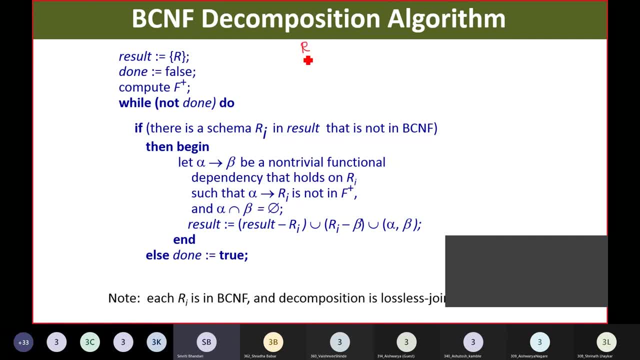 Right, So originally we are saying that we are having the relation R that we would like to decompose. Okay, So initially that relation R is assigned to our result. We are having one flag done That is assigned to false initially. 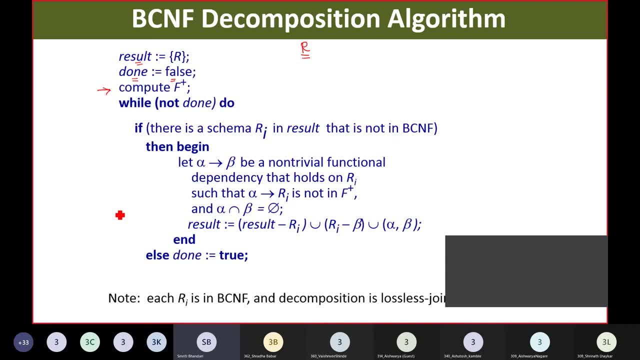 We are having computed our F+, We are having this iterative algorithm While not done due. so while this flag is not true, we are going to iterate through if there is a schema ri in result that is not in bcnf. so initially we are having only r and we know that this is. 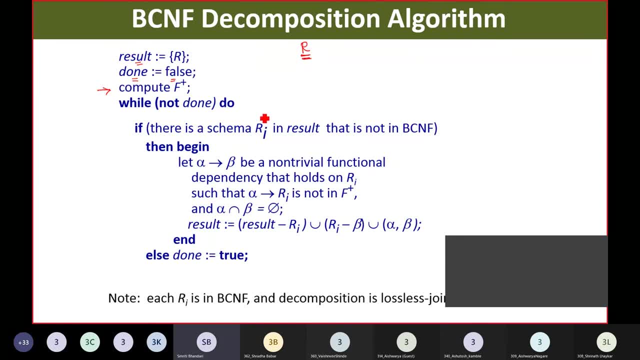 not in bcnf and that is why we are executing this algorithm. so if there is a schema ri in result that is not in bcnf, then what we need to do, we need to follow these steps. so we need to pick a functional dependency- alpha to beta- from this f plus, such that this dependency is non-trivial. 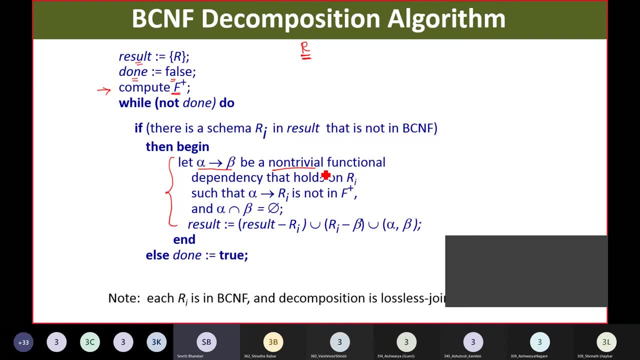 this dependency is non-trivial, right, and also this dependency dependency is not the super key of the relation ri under consideration. okay, i'll repeat: we need to test for two conditions. what are those two conditions? alpha to beta is non-trivial, because it is. if it is trivial, then it satisfies bcnf norm. so if alpha to beta is, 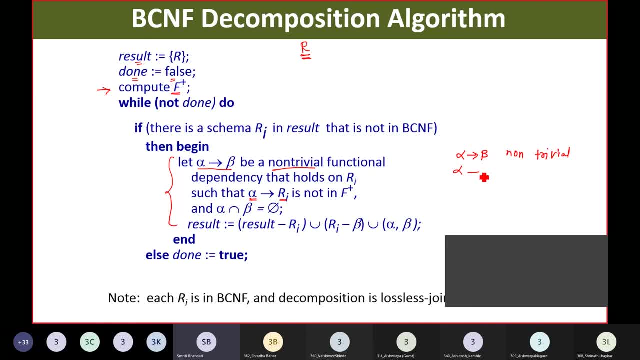 non-trivial and alpha is not the super key of ri, so alpha is not determining all the attributes of ri. right and alpha intersection. beta is phi. that means there is no common attribute in left hand side and right hand side of the relation. if these conditions are true, then for a particular dependency, alpha to beta. 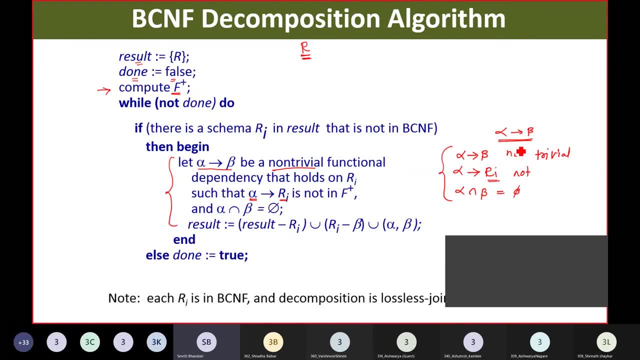 then we may say that this particular dependency is violating our norm. and that is why, by making use of this dependency, we are going to decompose our relation. and how we are going to decompose, see here the result is now. the new result is: result minus ri, union ri. minus beta, union alpha beta. what does this mean? whichever dependency that 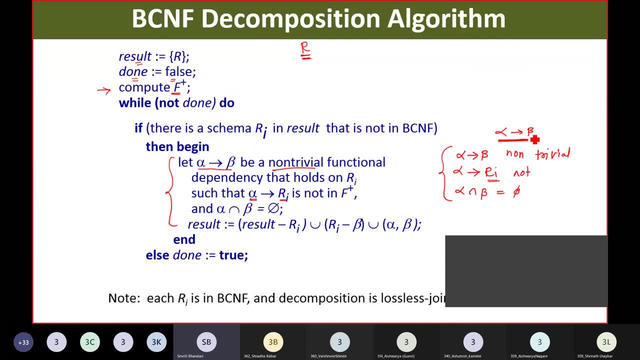 we have identified which is violating the norm of bcnf. we combine all those attributes together and we come up with a new relation. right another relation in the order of dc nf is equal to bc nf. right. Right Another relation would be: result: old result minus R i Okay, Union R i minus beta. 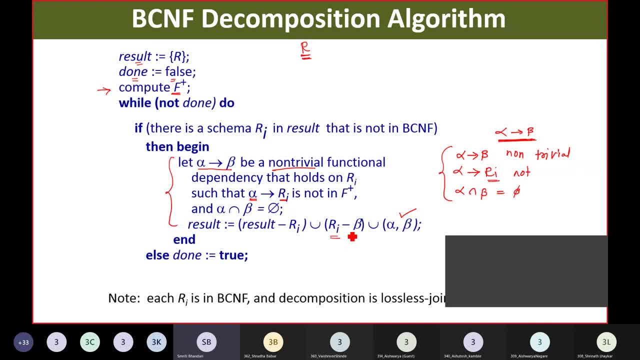 What does this mean? The relation under consideration, okay, minus the right-hand side, Minus the right-hand side of this functional dependency under consideration. So this will form only the left-hand side, or rather all the attributes other than this right-hand side of the dependency. So this will form one relation and combination of: 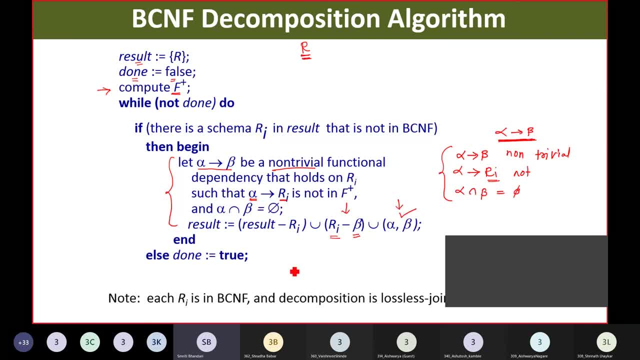 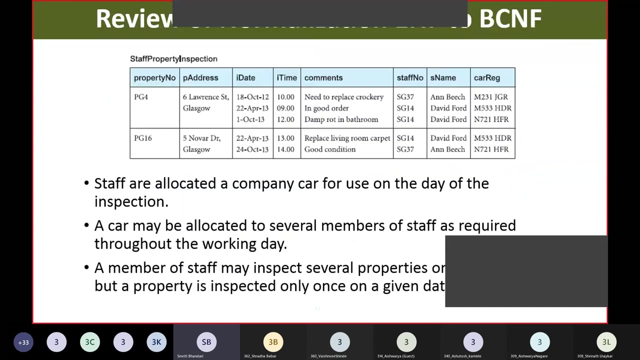 alpha beta will form another relation, Right. So these are the relations in our decomposition and we are going to iterate through Right Till we are finding such kind of a functional dependency that is violating the norm of BCNF. Okay. So I would suggest you to go through once again this algorithm and try to implement it. 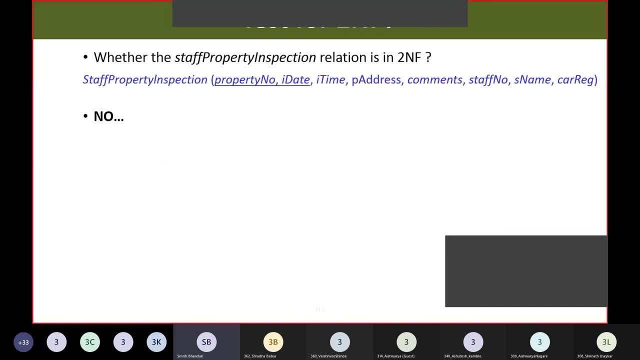 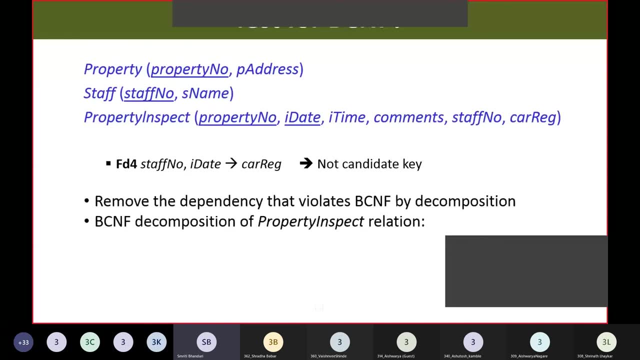 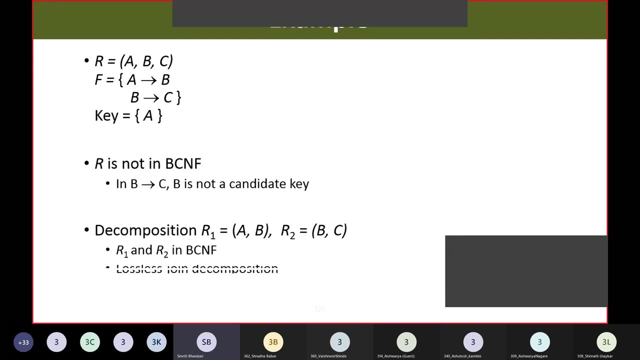 practically Okay. Now we are going to discuss one more case study, but right now I am omitting, I am skipping the discussion with respect to that case study. I will be, I will be posting this case study for you later so that you can go through. Okay, But now. 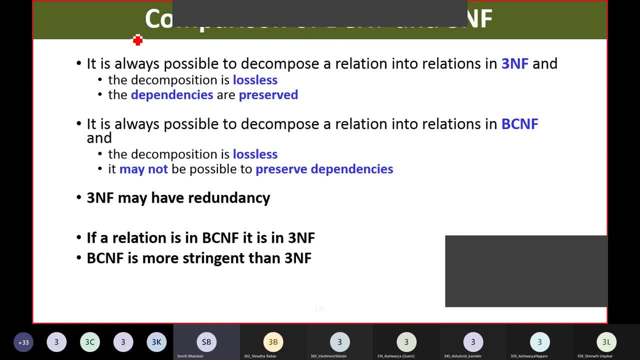 I will be comparing 3NF and BCNF and this is the most important comparison of BCNF and 3NF. So please remember these points. It is always possible to decompose a relation into relations in 3NF and the 3NF. decomposition is always lossless and preserving dependencies.